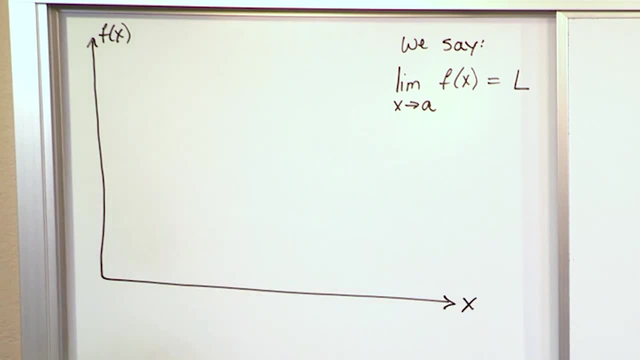 Now, when we do definition of a limit, it applies to any function f of x. So let's just draw some random function. So we'll do this something like this: Who knows what this function is, but it's some function of x. Notice that this particular one is smooth and continuous. 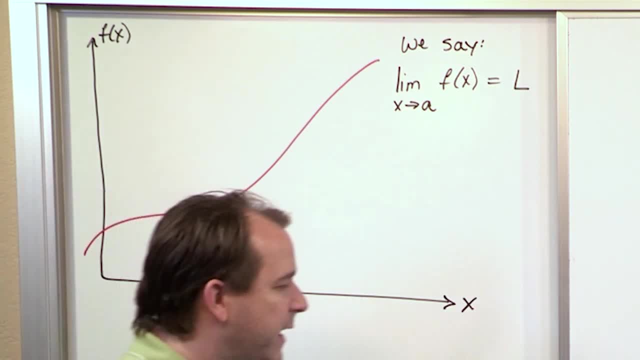 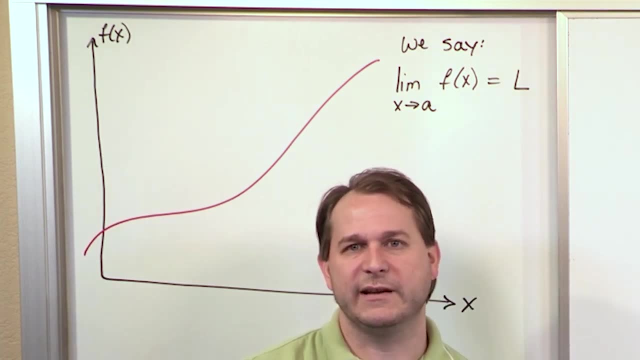 and we're just going to do that for now. But just keep in mind that for the limit to really exist, at a point we'll talk about more exactly what conditions the limit exists, But for now we're just going to say this guy's smooth and continuous, because it's easier to understand. 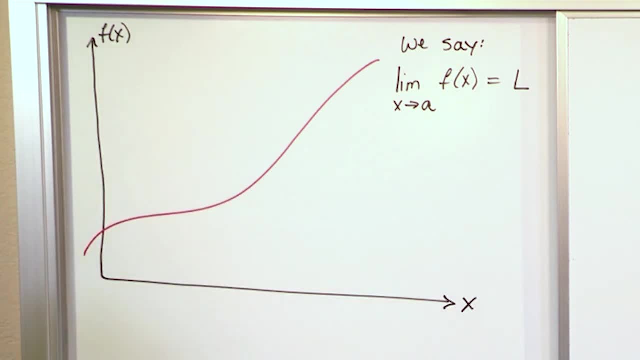 And then we say that notice, we said here as x approaches some number, a. So for the sake of argument let's say that a is right here. So we're trying to find, as x approaches the value, a. This could be three, like x approaches three, x approaches four, x approaches five, whatever. 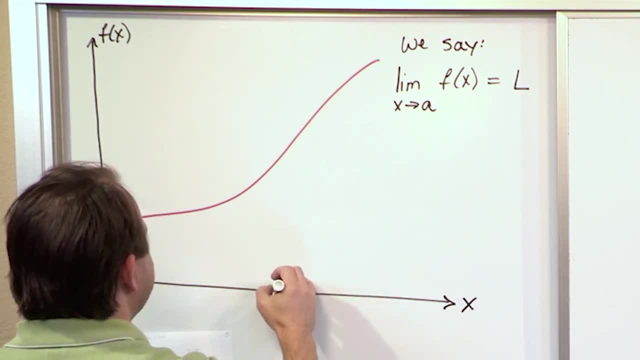 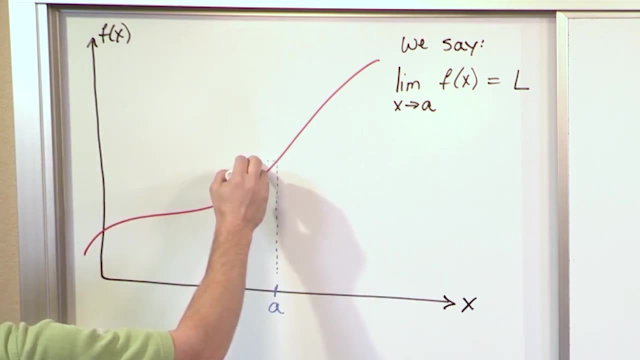 It's any value a, As x approaches some value a. so I'm going to actually go ahead and do a dotted line up here and let's see what the function actually says. So here's where the function is equal a And if you go across over here, you can see that the corresponding value of the function 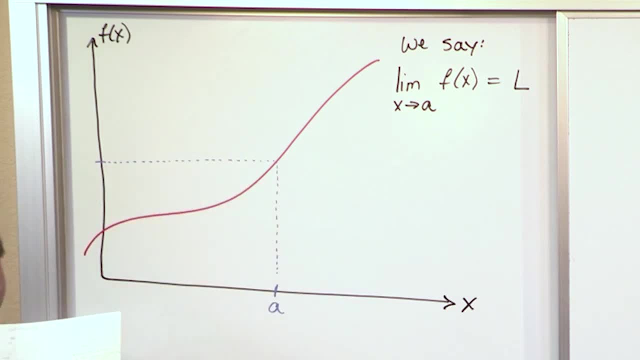 is listed right over here, And this value right here is what we call l. So what we're basically saying in a picture is: the limit as x approaches this value of a of this function is equal to l. It should be totally clear what we're trying to say, because we've been doing this over and over. 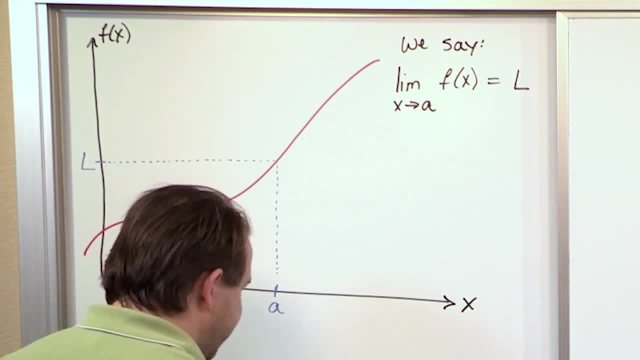 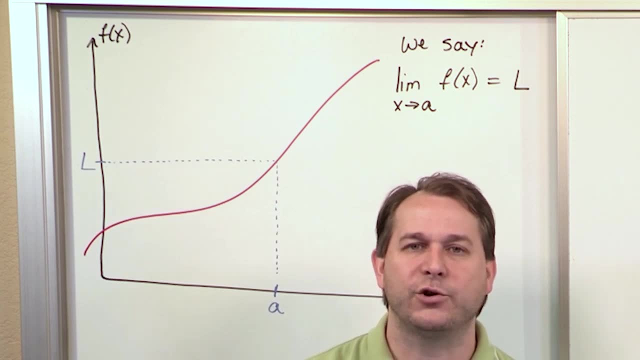 and over again. All right, Now, when we define the definition of the limit, we have to introduce some additional ideas, because, you've got to remember, the definition of this limit is a mathematical proof. You see, I've already told you that limits exist under certain conditions. I've 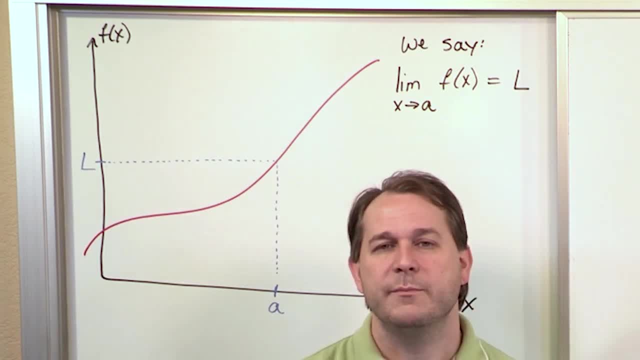 already told you, you get infinitely close to it. I've already told you all these things, But really in math you can't just tell somebody in layman's terms what it is. You have to construct some sort of framework, some sort of proof that shows that these limits exist for every possible function. 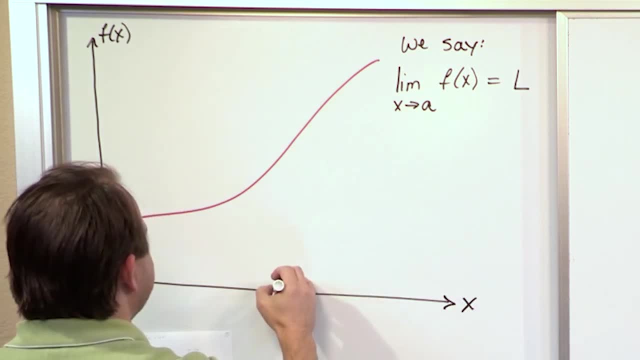 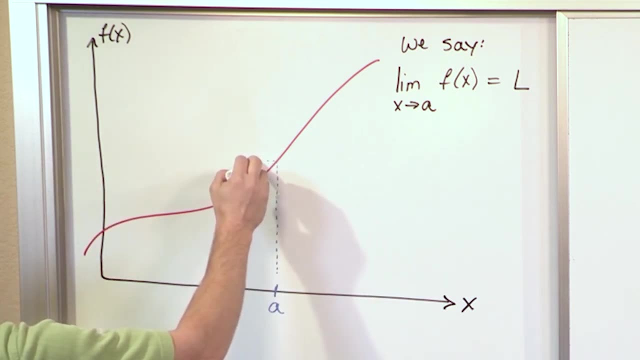 It's any value a As x approaches some value a. so I'm going to actually go ahead and do a dotted line up here and let's see what the function actually says. So here's where the function is at. that value x equals a. So I'm going to actually go ahead and do a dotted line up here. 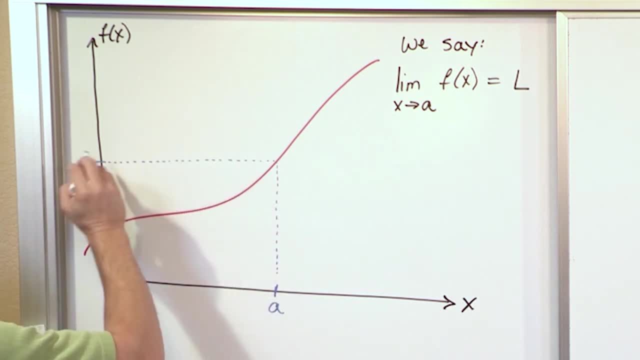 x equals a And if you go across over here, you can see that the corresponding value of the function is listed right over here And this value right here is what we call l. So what we're basically saying in a picture is the limit as x approaches. this value of a of this function is. 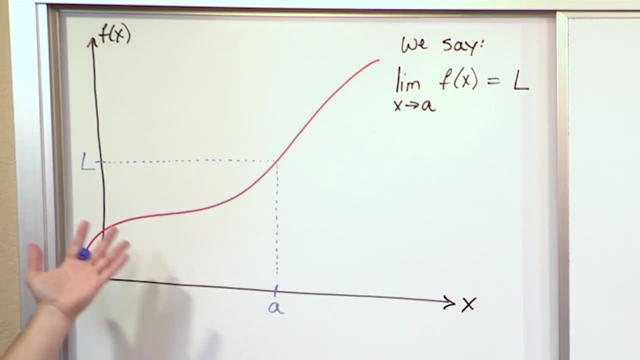 equal to l. It should be totally clear what we're trying to say, because we've been doing this over and, over and over again. Now, when we define the definition of the limit, we have to introduce some additional ideas because, you've got to remember, the definition of this limit is a. 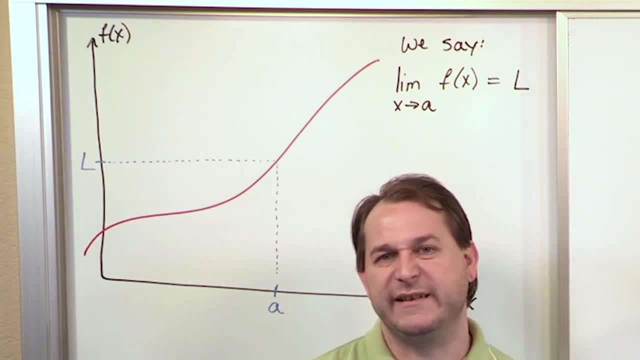 mathematical proof. You see, I've already told you that limits exist under certain conditions. I've already told you you get infinitely close to it. I've already told you all these things. But really in math you can't just tell somebody in layman's terms what it is. You have to construct some sort 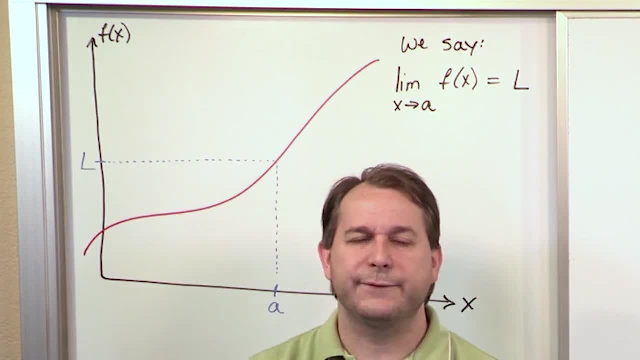 of framework, some sort of proof that shows that these limits exist for every possible function, that we could draw on the board, or at least have some methodology that we could then use to find any limit we want. okay, So it's not enough just to draw this here. We have to have a few more. 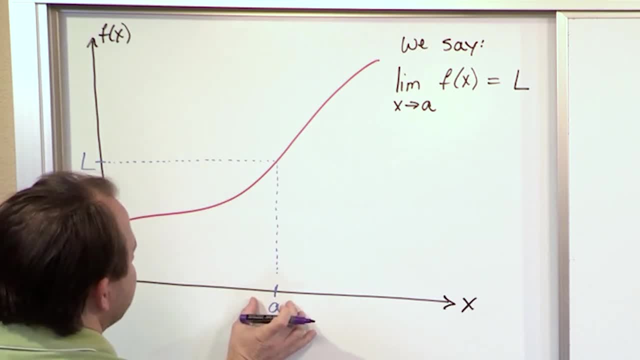 ideas. So we're going to introduce something here. So here is the x approaching a, But of course, as you get closer and closer and closer to a, you're going to approach that limit. But let's introduce a value close to a on this side and a value close to a over here, because, as you know, 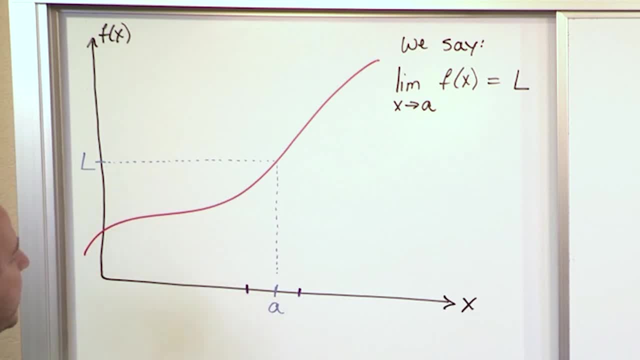 you can approach the limit from this direction, approach the limit from this direction. You know, as we were doing our table of values, we could plug in values on either side of a and get closer and closer and closer. So we'll pick some values close by And this value here. 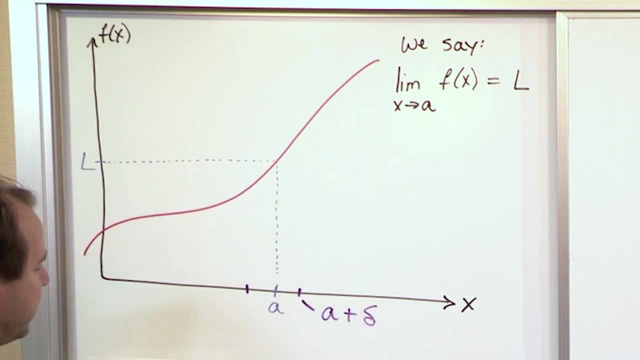 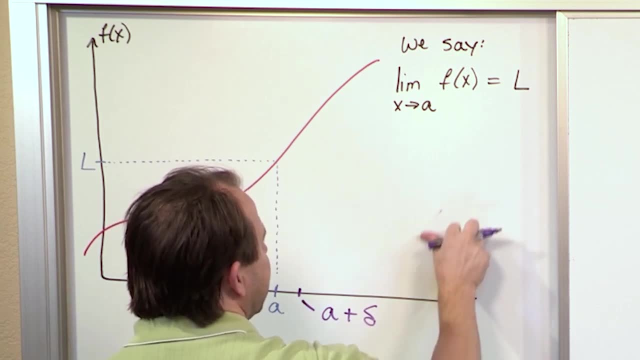 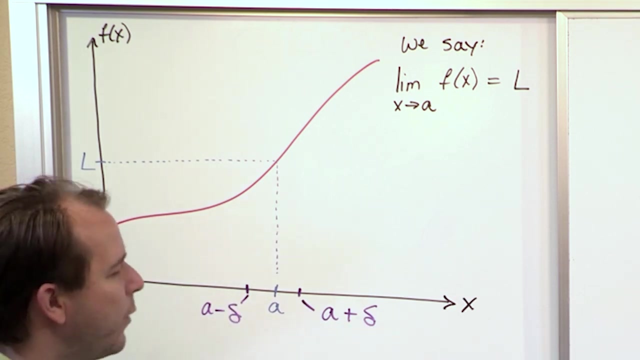 we'll call a plus some number delta. This is a lowercase delta. You might have seen the triangle as the uppercase delta. Well, this is just a lowercase Greek letter delta. okay, And then this one is a minus some number delta. Do not worry about what delta means For now, just know. 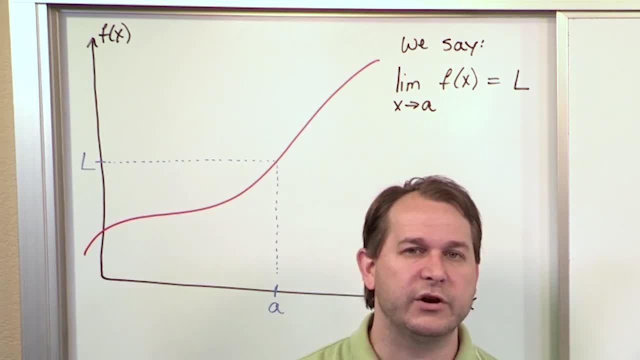 that we could draw on the board or at least have some methodology that we could then use to find any limit we want. Okay, So it's not enough just to draw this here. We have to have a few more ideas. So we're going to introduce something here. So here is the x approaching a, But of course, 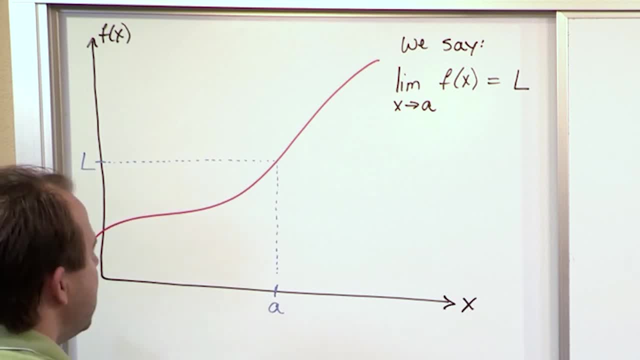 as you get closer and closer and closer to a, you're going to approach that limit. But let's introduce a value close to a on this side and a value close to a over here, Because, as you know, you can approach the limit from this direction, approach the limit from this direction. 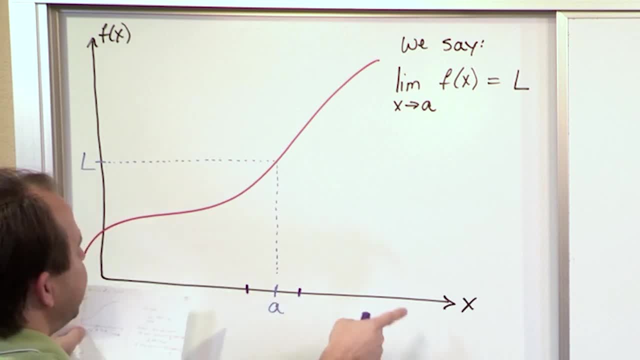 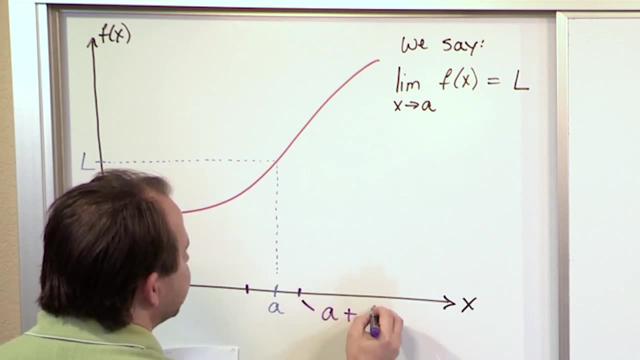 You know, as we were doing our table of values, we could plug in values on either side of a and get closer and closer and closer. So we'll pick some values close by And this value here we'll call a plus, some number delta. This is a lowercase delta. You might have seen the triangle. 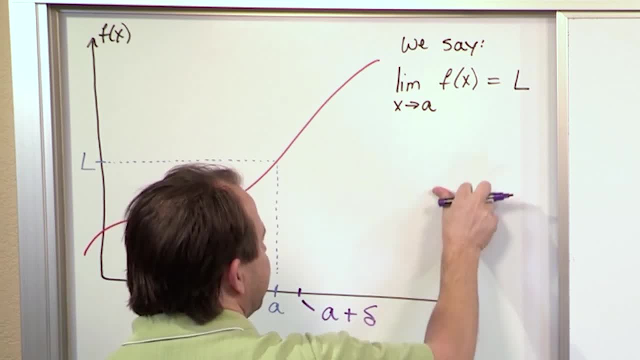 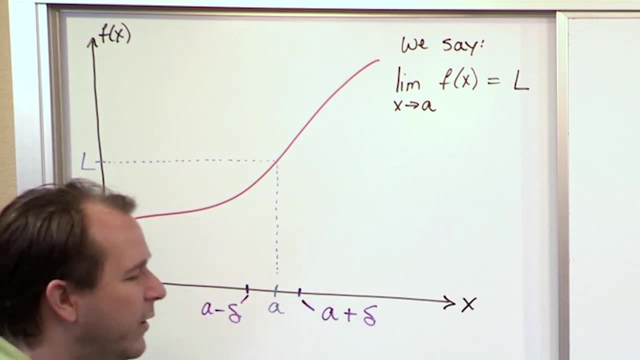 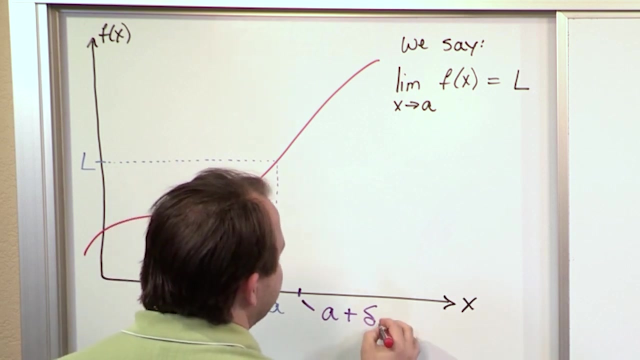 as the uppercase delta. Well, this is just a lowercase Greek letter, delta. Okay, And then this one is a minus some number, delta. Do not worry about what delta means, For now, just know that delta is a small number, a teeny, weeny number. So I'm going to put a little. 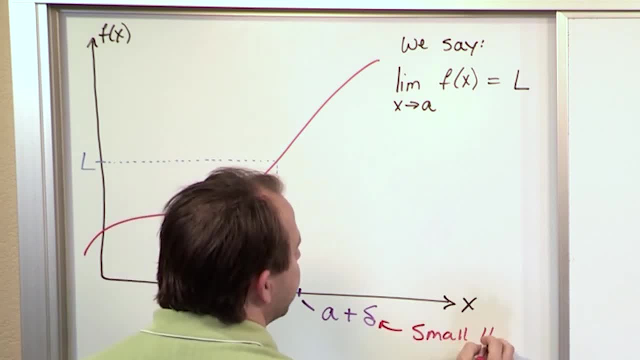 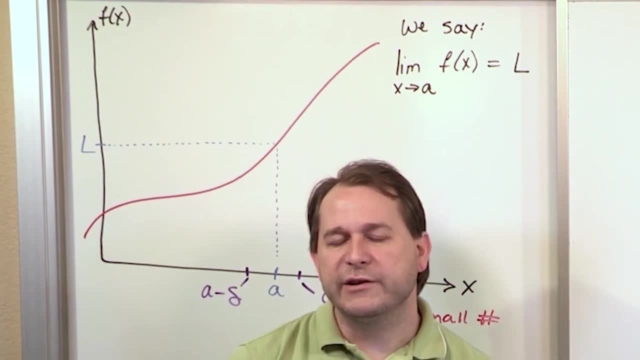 row here. Delta is just a small number And I'll give you a little bit of a preview. Why do you think we're doing this? a minus delta and a plus delta? Because, ultimately, what we're really trying to say when we define a limit is that you get closer and closer and closer to the value of a. 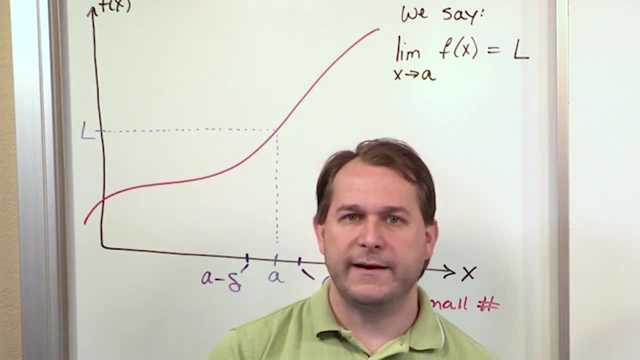 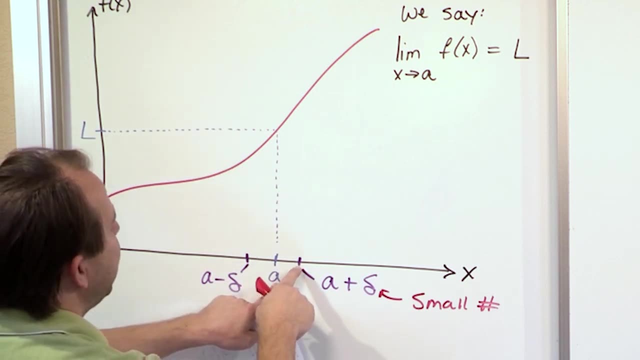 without ever getting to a. That's the layman term way of explaining it to you. And now you know that you've been knowing that for a long time. But mathematically, what you do is you say, hey, we want to get closer to a, So what we'll do is we'll pick a value over here. That's a plus a. 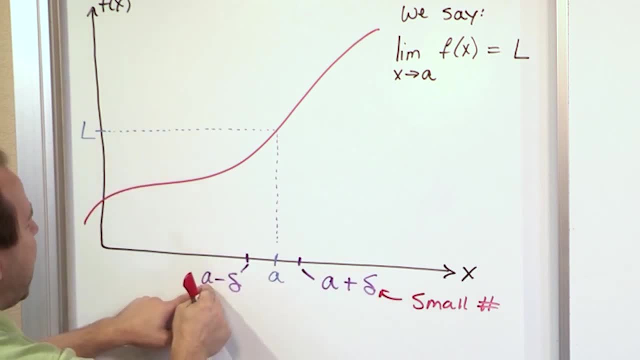 teeny weeny number And we'll pick a value over here. that's a minus, starting with a minus a teeny weeny number. So this difference here, this value here, between a and these marks, this is a tiny number called delta And ultimately we're going to let delta get really, really, really small, which is going: 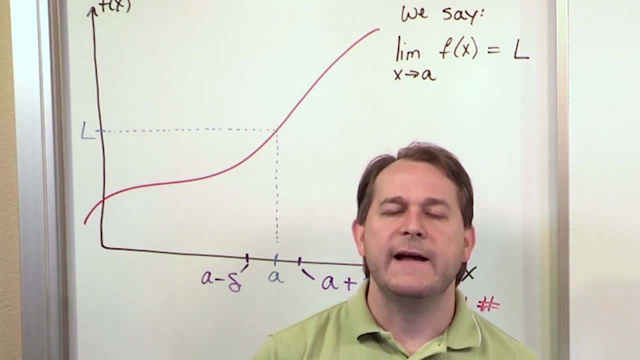 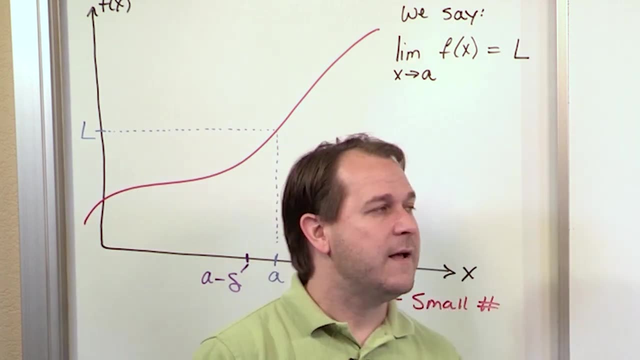 to let us approach the value of a and get infinitely close to a. The delta thing is just a mechanism to allow us to approach a and get very, very close to it without ever getting there, And you'll see this pop up in the definition. 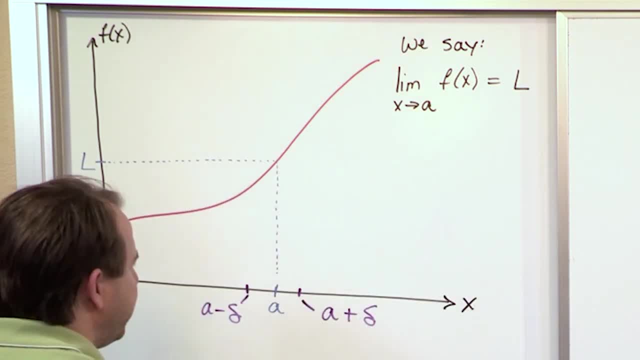 that delta is a small number, a teeny, weeny number. So I'm going to put a little arrow here. Delta is just a small number And I'll give you a little bit of a preview. Why do you think we're doing this? a minus delta and a plus delta, Because, ultimately, what we're really trying to 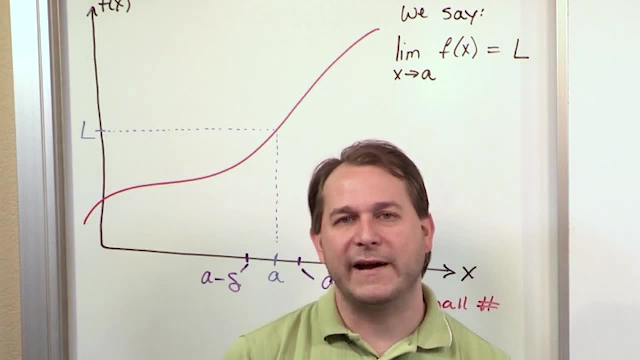 say, when we define a limit is that you get closer and closer and closer to the value of a without ever getting to a. That's the layman term way of explaining it to you. And now you know that. You've been knowing that for a long time. But mathematically what you do is you say, hey, we want. 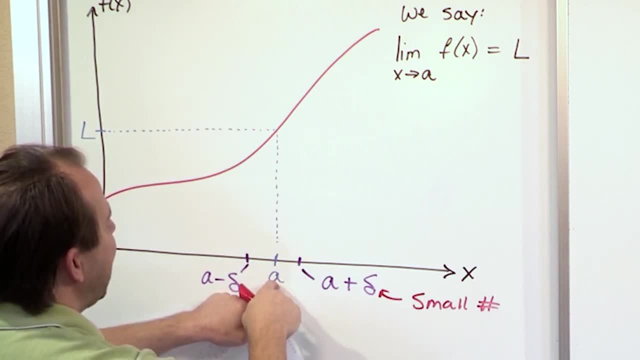 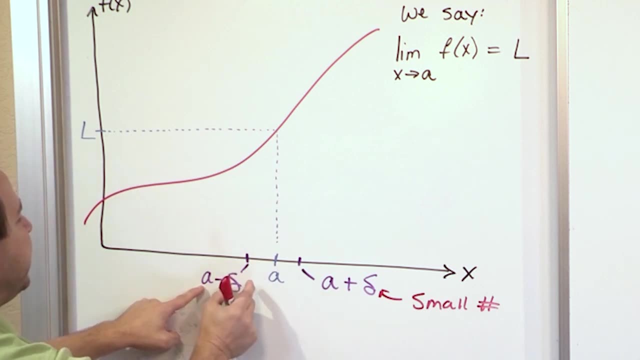 to get closer to a. So what we'll do is we'll pick a value over here- that's a plus- a teeny weeny number- And we'll pick a value over here- that's a minus. so, starting with a minus, a teeny weeny. 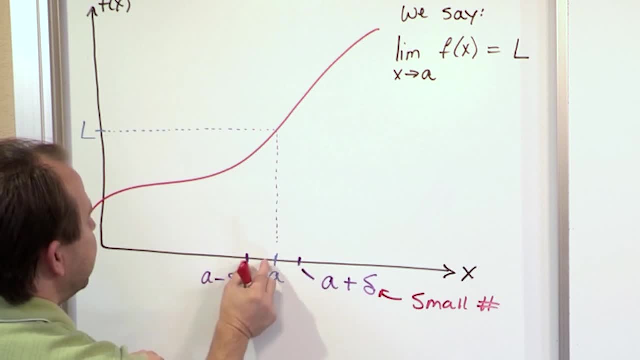 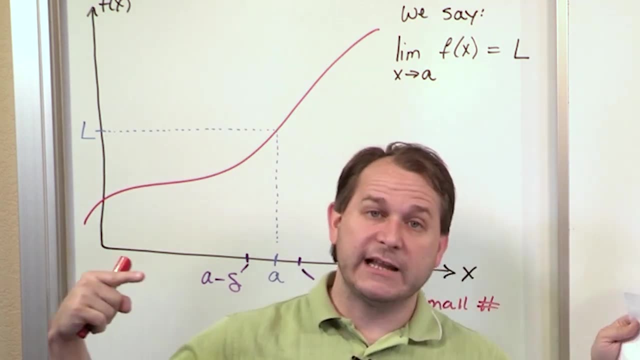 number. So this difference here, this value here, between a and these marks, this is a tiny number called delta And ultimately, we're going to let delta get really, really, really small, which is going to let us approach the value of a and get infinitely close to a. That's the delta thing. 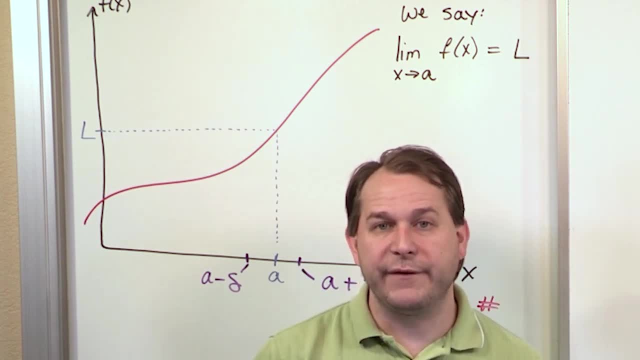 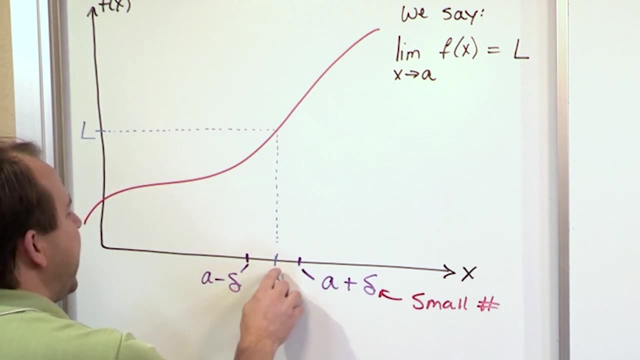 It's just a mechanism to allow us to approach a and get very, very close to it without ever getting there, And you'll see this pop up in the definition. okay, But anyhow, if this is a very small value to the right of a and this is a very small value to the left, 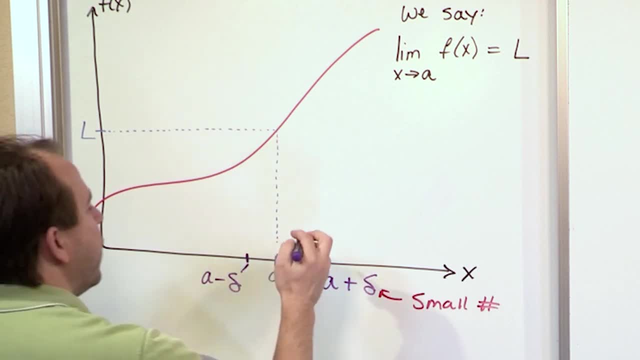 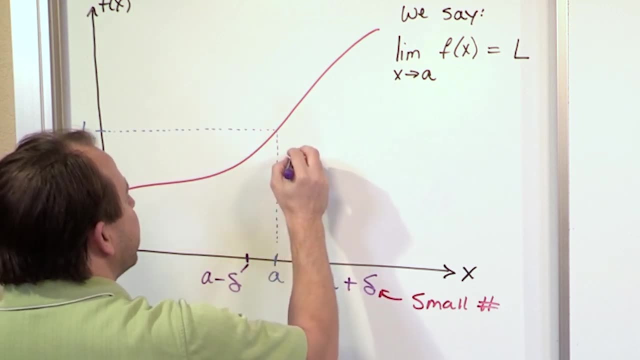 of a. what do you think is going to happen if I go up here? What would the value of the function be? that would correspond to this value of x, Because this is just a little bit to the right. Well, I can, of course, go up to this guy here And I see that it intersects the function over. 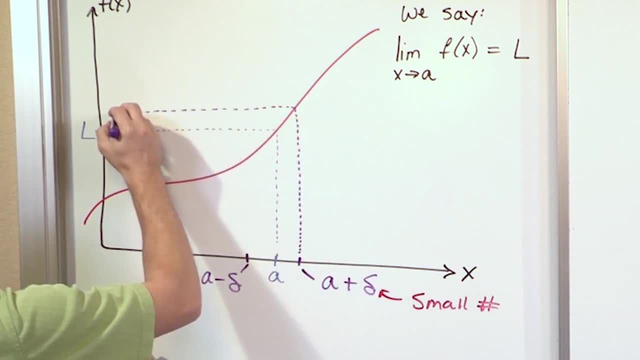 there And I can go over here and see where it intersects right there. okay, So obviously it's intersecting the f of the axis here at a value Larger than l. okay, So what we do is we label this l plus some other small number- epsilon, This: 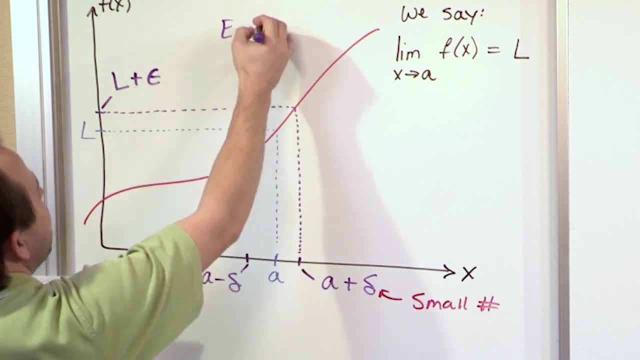 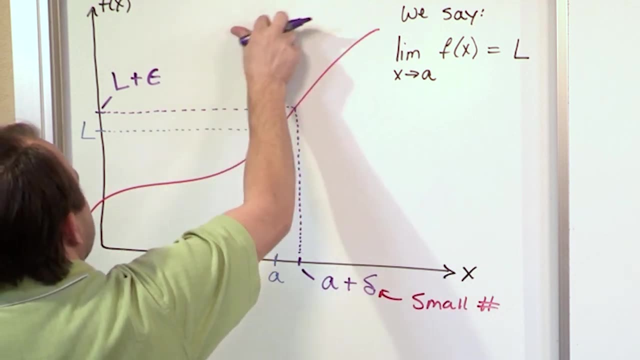 looks like a kind of a curved e. Instead of, you know, like an e like this, you make a curve like a c And then you put a little thing in the middle That is a very small number called epsilon. So we remember that. Now we have another corresponding value very close to a. But on 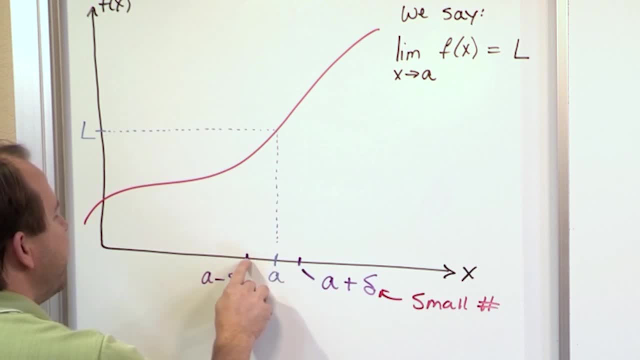 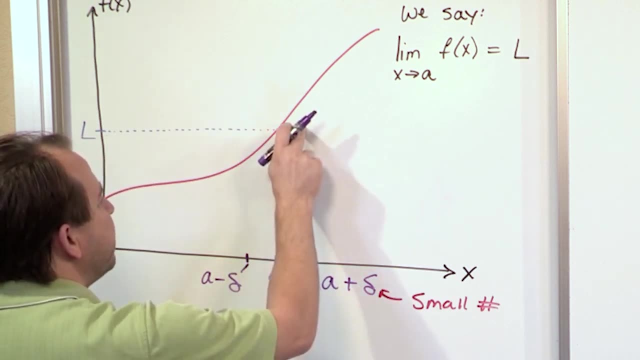 But anyhow, if this is a very small value to the right of a and this is a very small value to the left of a, what do you think is going to happen? if I go up here, What would the value of the function be that would correspond to this value of x. 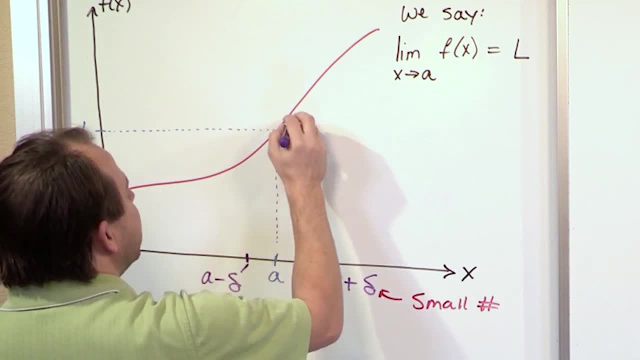 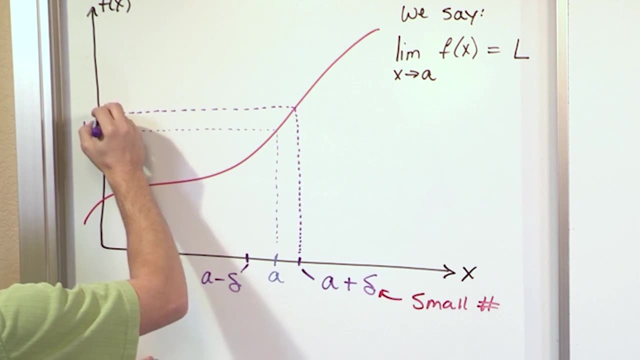 because this is just a little bit to the right. Well, I can of course go up to this guy here and I see that it intersects the function over there, And I can go over here and see where it intersects right there. Okay, So obviously it's intersecting the f of the axis here at a value —. 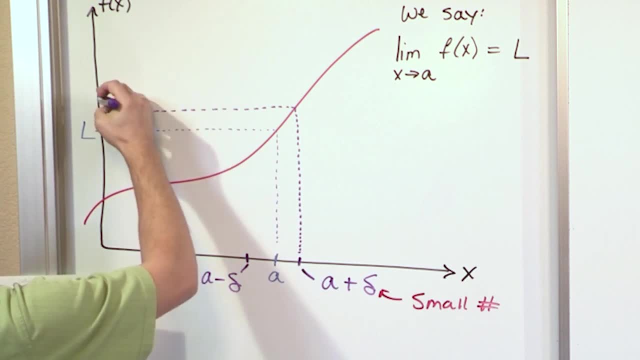 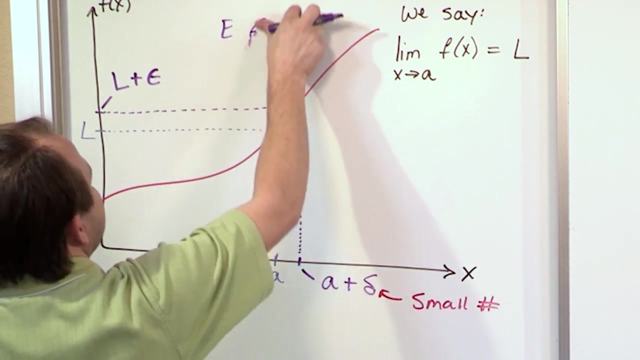 you larger than L. okay, So what we do is we label this L plus some other small number, epsilon. This looks like a kind of a curved E. Instead of, you know, like an E, like this, you make a curve like a C and then you put a little thing in the middle That is a very small number called epsilon. So 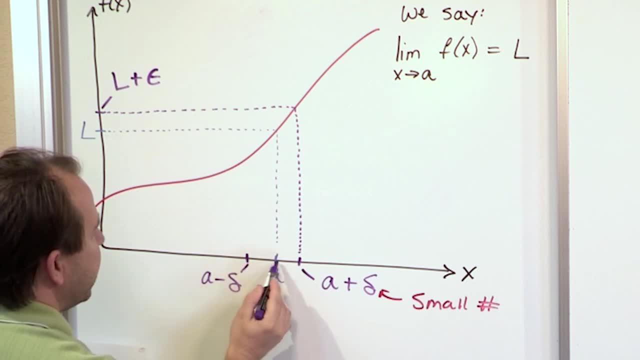 we remember that Now we have another corresponding value very close to A. but on the left-hand side we can do the same kind of thing. We can go up here, we intersect the function and we see where the corresponding value is over here And it intersects right here. So then we can draw a. 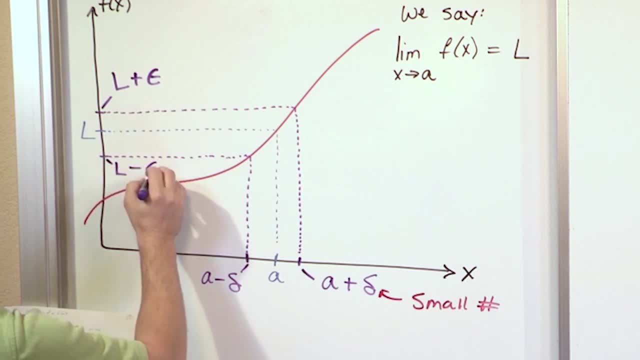 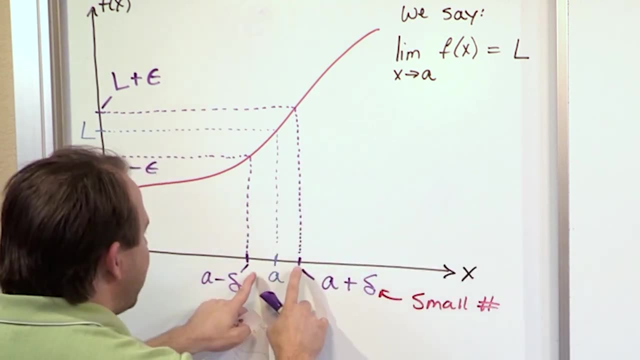 little line here and remind ourselves that this is L minus some tiny, tiny number called epsilon. Now I'm drawing everything large on the board so that you can see it. but really, this value, A plus delta and A minus delta, these two values, they're really, really, really, really really. 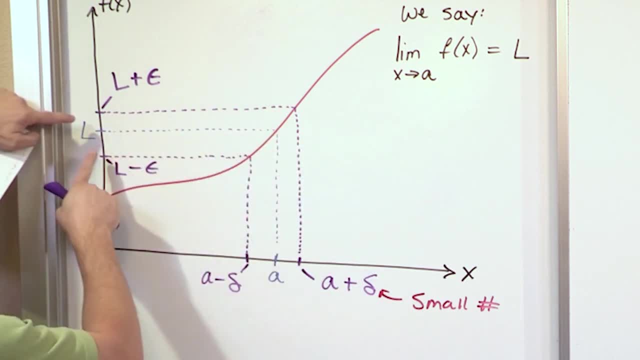 close to A, okay, And because of that, the corresponding values of the function that correspond to those are really really, really close to L. One of them is a little bit higher than L, just a little bit higher by the small number, epsilon, And this guy is just a. 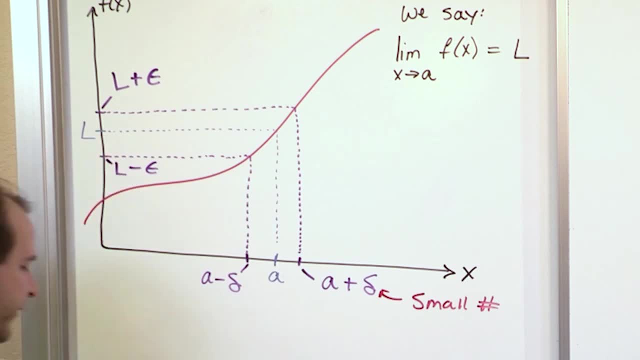 little bit lower than L, just a little bit lower by a small number called epsilon. So again, this number here is a small number. The only real takeaway I want you to get from this is that delta is a very small number. In fact, we're going to let it become infinitely small. 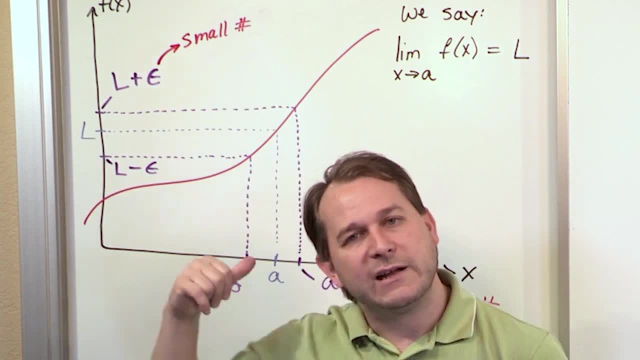 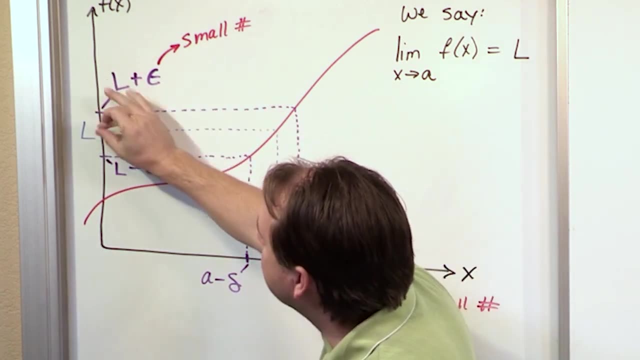 as we approach X, X approaches A, And we're going to allow epsilon because of the way it's drawn here. you can see that as these two guys get closer and closer, these are going to get closer and closer, So epsilon becomes a very, very small number as well. So the takeaway that 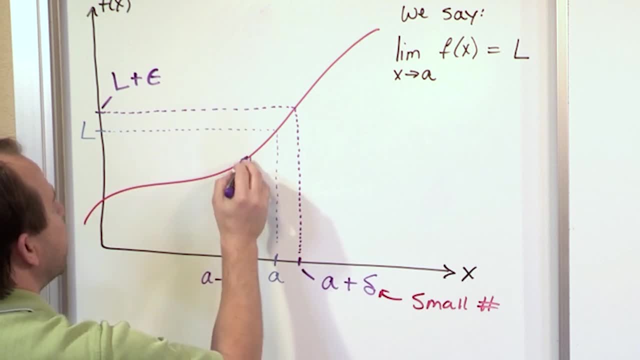 the left-hand side we can do the same kind of thing. We can go up here, We intersect the function, We can see where the corresponding value is over here And it intersects right here. So then we can draw a little line here and remind ourselves that this is l minus some tiny, tiny number called. 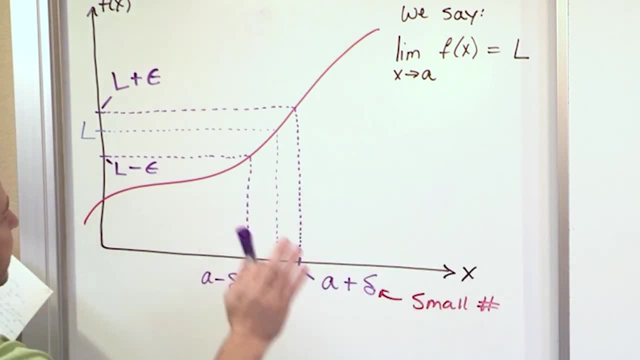 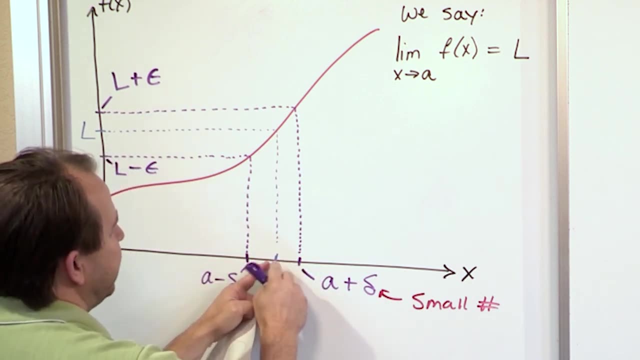 epsilon. Now I'm drawing everything large on the board so that you can see it. But really, this value, a plus delta and a minus delta, these two values, they're really, really, really, really, really close to a okay And, because of that, the corresponding values of the function. 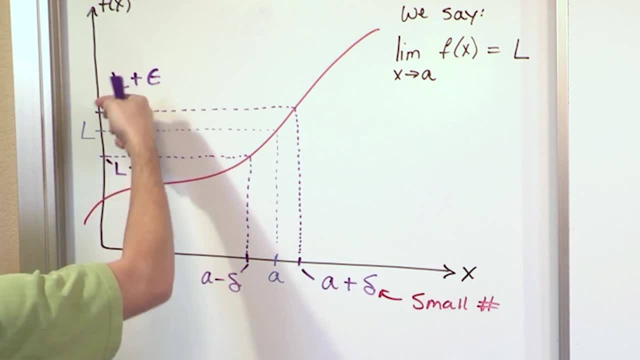 that correspond to. those are really, really, really close to l. One of them is a little bit lower than l, just a little bit higher by the small number epsilon. And this guy is just a little bit lower than l, just a little bit lower by a small number called epsilon. So again, 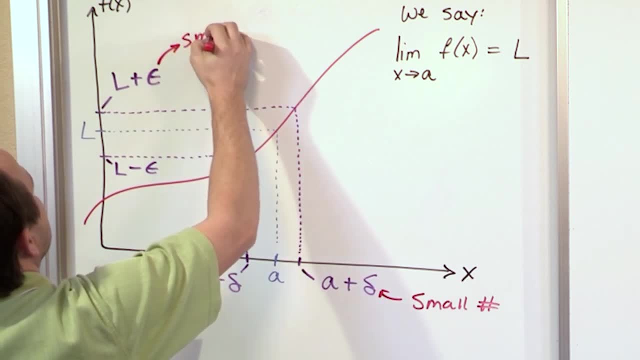 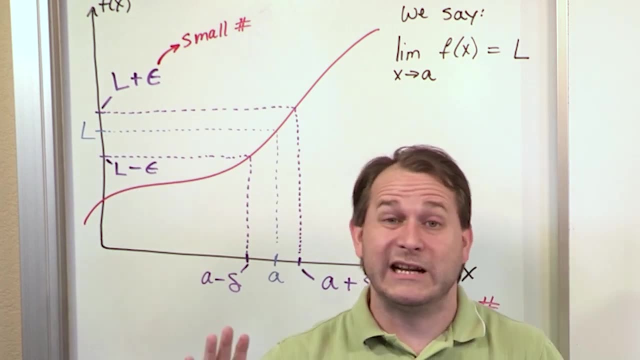 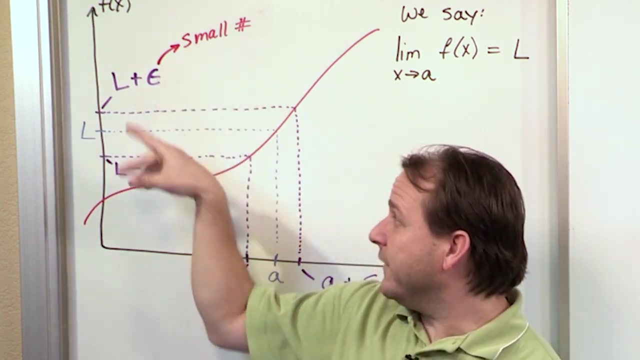 this number here is a small number. The only real takeaway I want you to get from this is that delta is a very small number. In fact, we're going to let it become infinitely small as we approach x, approaches a, And we're going to allow epsilon because of the way it's drawn. 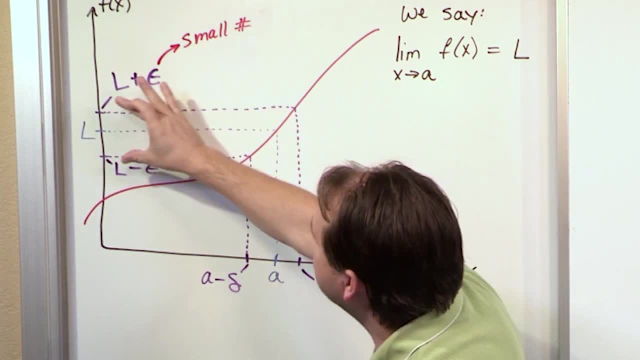 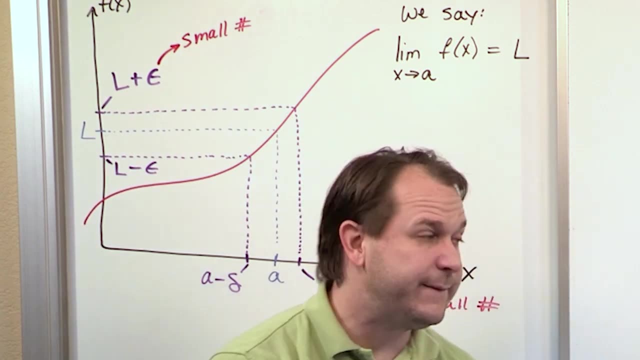 you can see that as these two guys get closer and closer, these are going to get closer and closer, So epsilon becomes a very, very small number as well. So the takeaway that I want you to see from here, okay, is something I'm going to write on the board here, And it's something that you can. 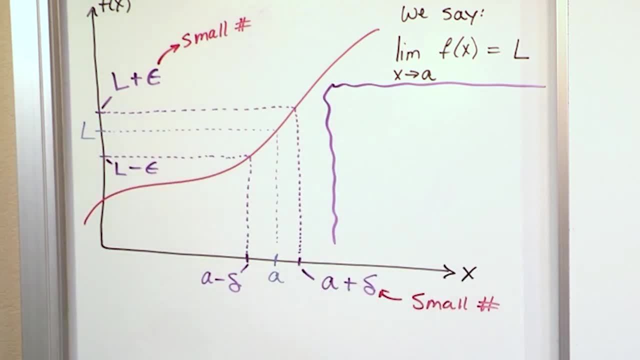 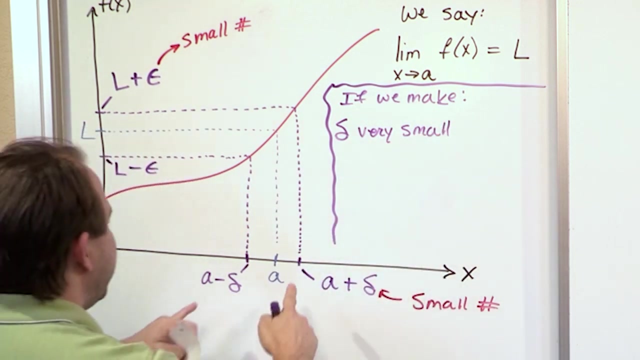 see from the drawing, but I want to make sure to write it down. Okay, if we make delta vary small, what is that going to do? What's going to basically happen is these points: if we make delta really, really small, these points are going to get closer and closer, and 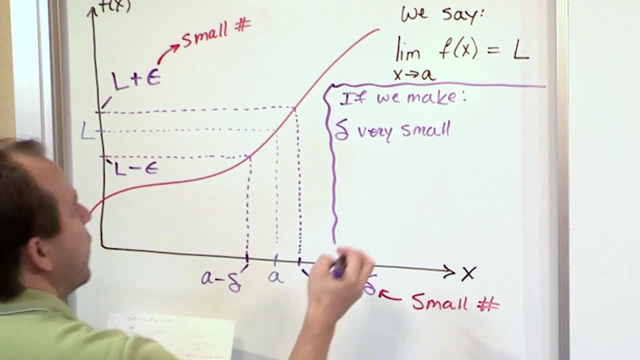 closer and closer to a. That's what's going to happen. What we're going to say is that x is going to approach a. So this is the mechanism that allows us to take our test value as we plug it in our table or whatever, and it gets infinitely close to a Making delta. 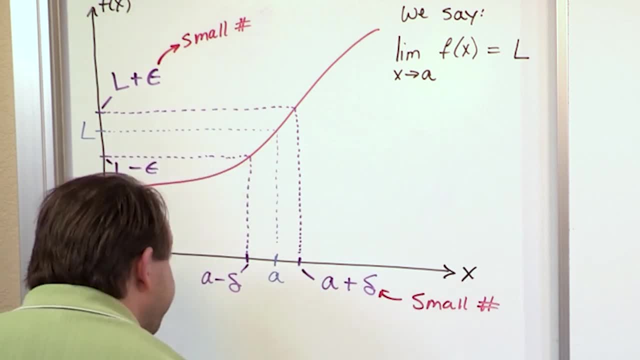 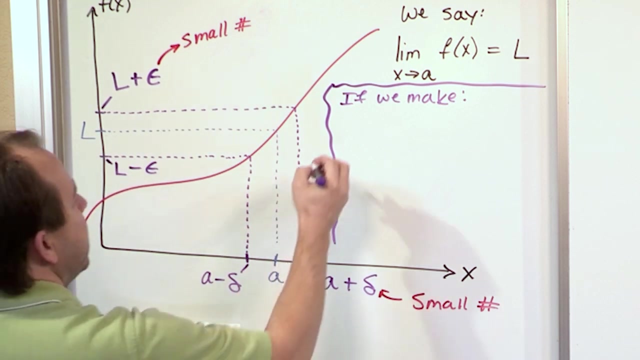 I want you to see from here. okay is something I'm going to write on the board here And it's something that you can see from the drawing, but I want to make sure to write it down. Okay, if, if we make, if we make delta very. 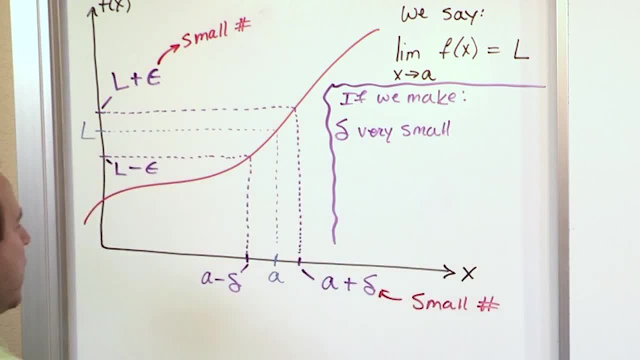 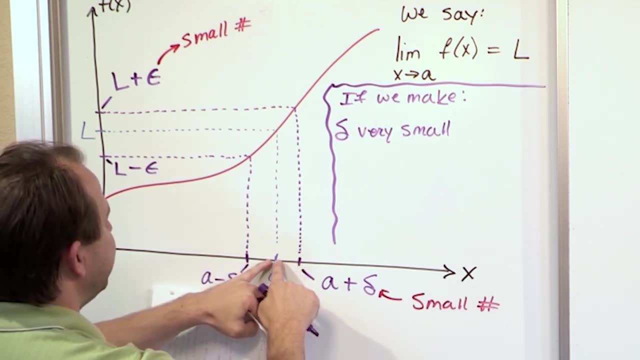 small. what is that going to do? What's going to basically happen is these points: if we make delta really, really small, these points are going to get closer and closer and closer and closer to A. That's what's going to happen. What we're going to say is that X is going to approach A, So this: 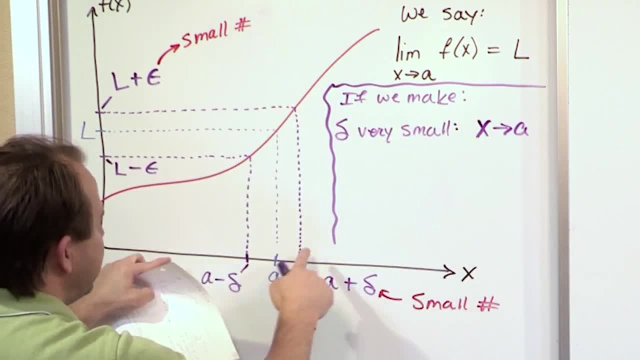 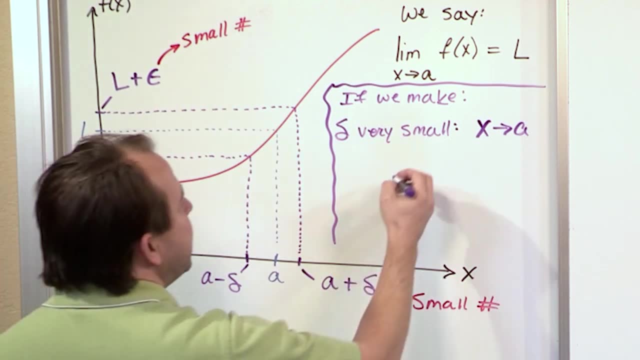 is the mechanism that allows us to take our test value as we plug it in our table or whatever, and it gets infinitely close to A Making. delta small is just basically the mechanism that does that, And then I'm going to draw a little arrow. 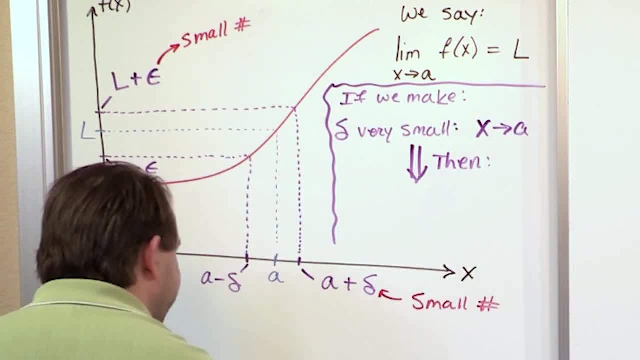 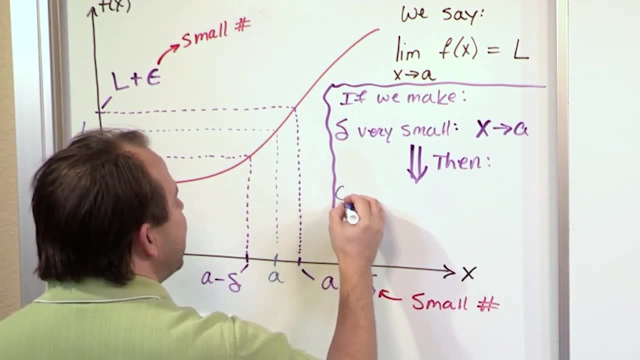 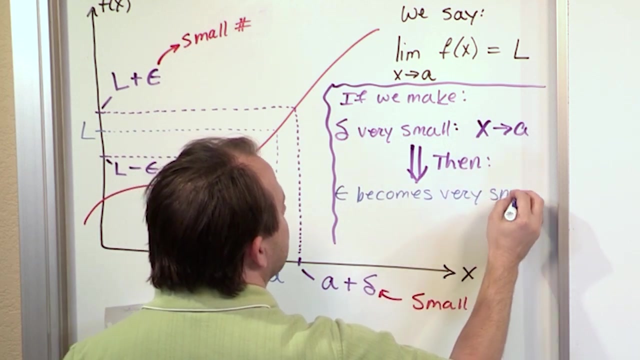 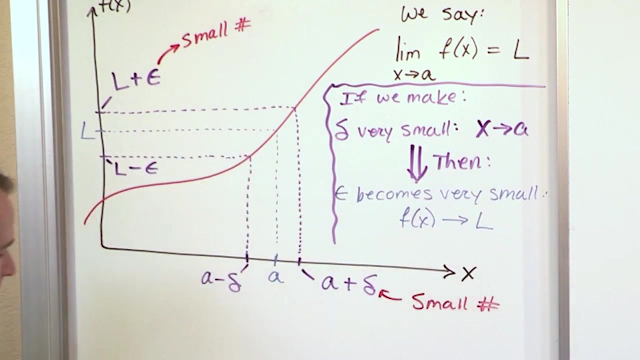 and then I'm going to say then- and I'll switch colors just to break it up: as a consequence of making this guy get closer and closer to A, what happens then is that epsilon becomes very small, And what that means is that F of X approaches the limit L. Okay. so ultimately what? 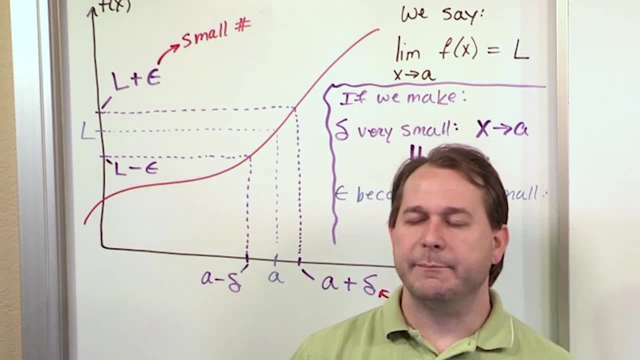 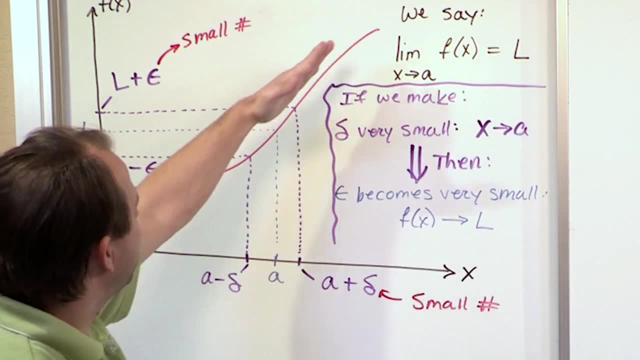 I've drawn on the board really is the entire definition of a limit, but it's done graphically and it's done without a lot of words, but it's just a concept, and that concept is saying: we have some function here, the red line, okay, we. 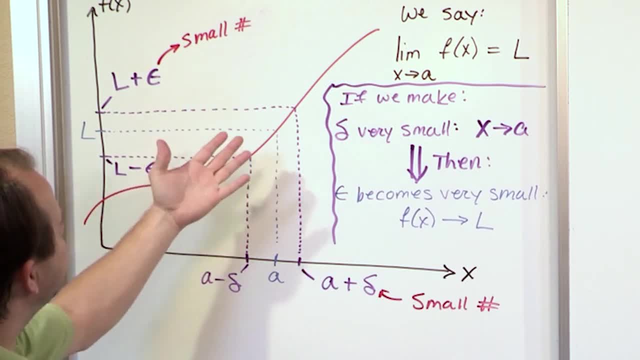 want to approach a. we want to get infinitely closer a and you can see from the drawing that, as we get infinitely close to a, what's going to happen is the function is going to get infinitely close to the, to the limit l, and we say that in math, that the limit as x approaches a of the. 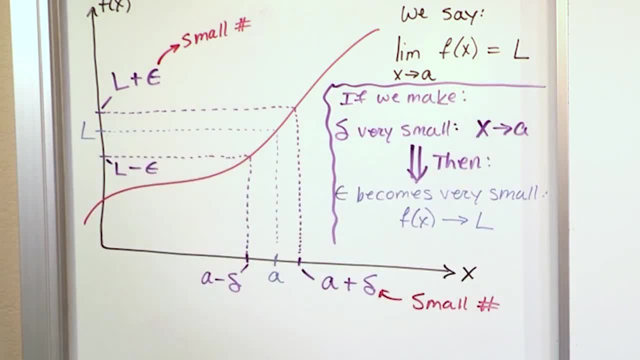 function f of x is equal to l and that's 100. true, okay, but the way that we actually pull it off mechanically in the framework of mathematics is we have to set a framework up, and what we do is we say: okay, we want to get closer and closer to this, so we'll pick a value to the right of. 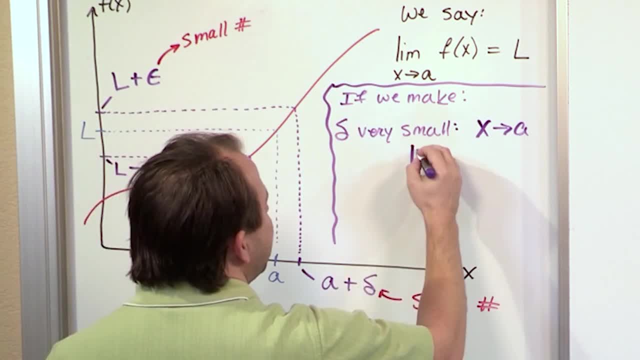 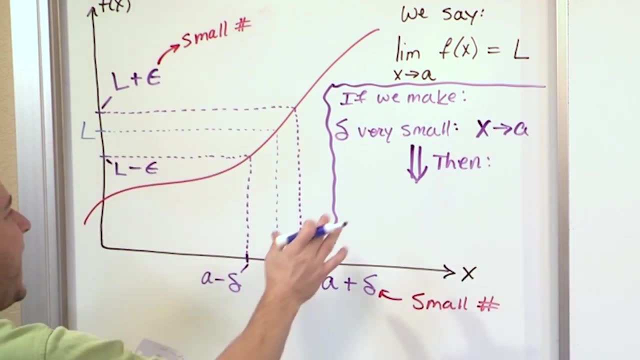 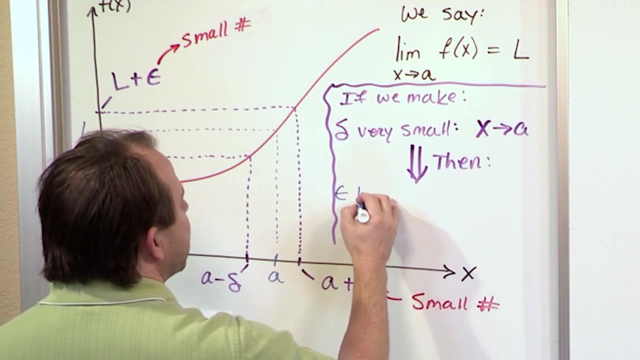 small is just basically the mechanism that does that, And then I'm going to draw a little arrow and then I'm going to say then, and I'll switch colors just to break it up- as a consequence of making this guy get closer and closer to a, what happens then is that epsilon becomes. 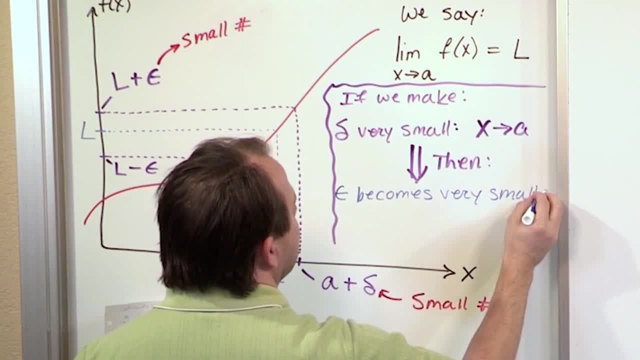 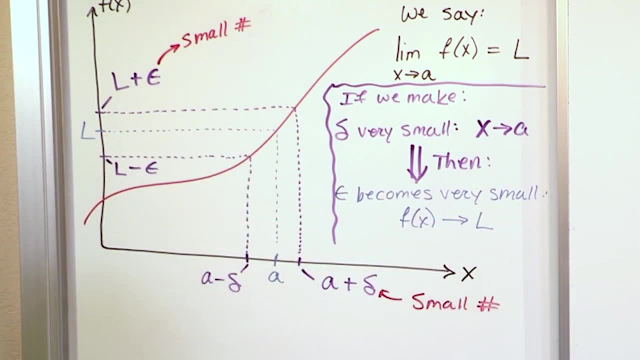 very small, And what that means is that f of x approaches the limit l Okay. so, ultimately, what I've drawn on the board really is the entire definition of a limit, But it's done graphically and it's done without a lot of words. 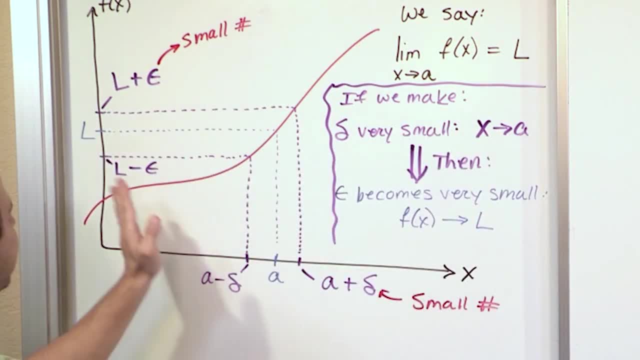 but it's just a concept, And that concept is saying: we have some function here, the red line. We want to approach a. we want to get infinitely close to a and you can see from the drawing that, as we get infinitely close to a, what's going to happen is the function is going to get infinitely. 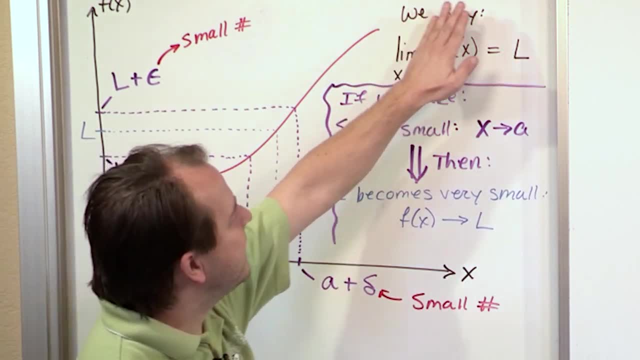 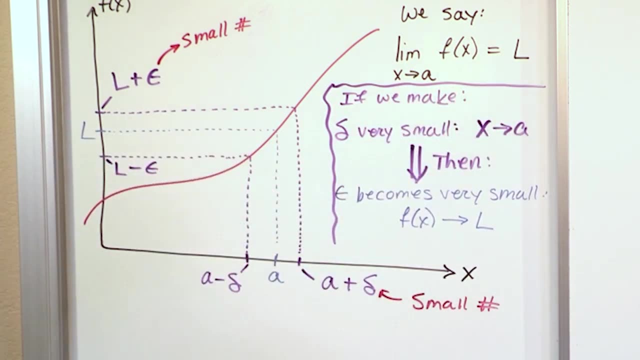 close to the limit l. And we say that in math, that the limit as x approaches a of the function f of x is equal to l, And that's a hundred percent true. Okay, but the way that we actually pull it off mechanically in the framework of mathematics is we have to set 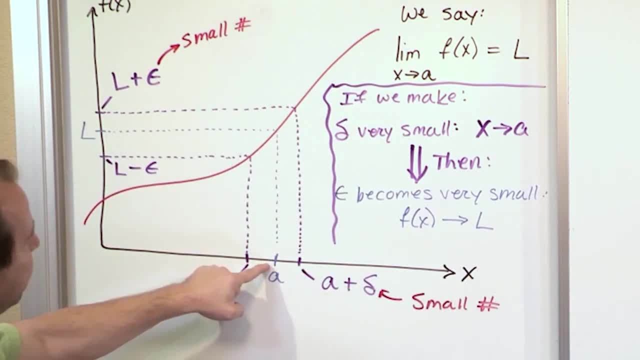 a framework up, And what we do is we say, okay, we want to get closer and closer to this, So we'll pick a value to the right of this and we'll pick a value to the left of this, And the value only. 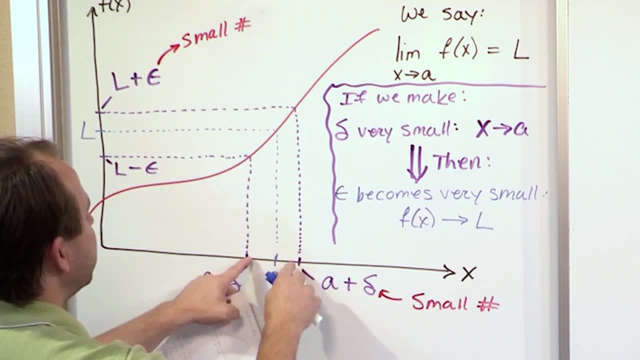 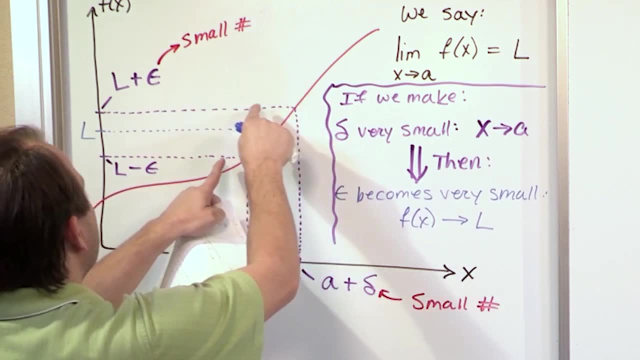 differs by this tiny, tiny number that we call delta. Both of these points are equidistant on this side, to the left and to the right, by a tiny, tiny thing: delta. Okay now, as the drawing stands, these correspond to values up here, one of which is a little bit higher and a little bit lower than. 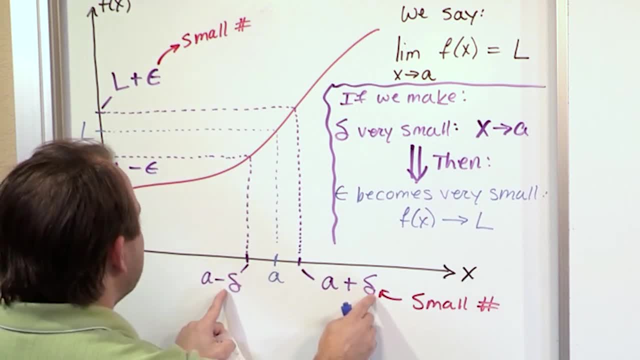 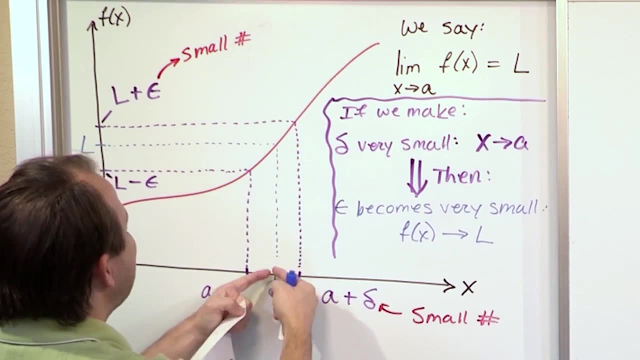 the limit that we're seeking l, But what we're going to do is we're going to make delta get very, very small. So what's going to happen is we're going to encroach closer and closer and closer and get infinitely close to. 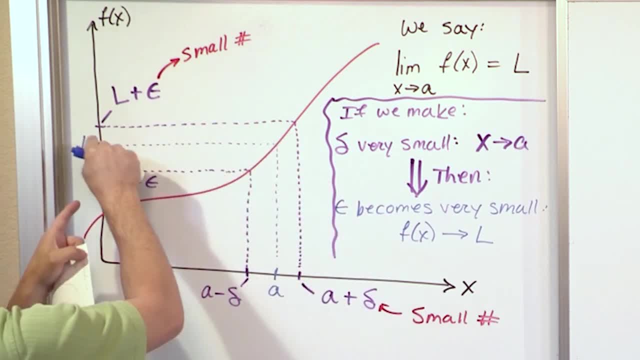 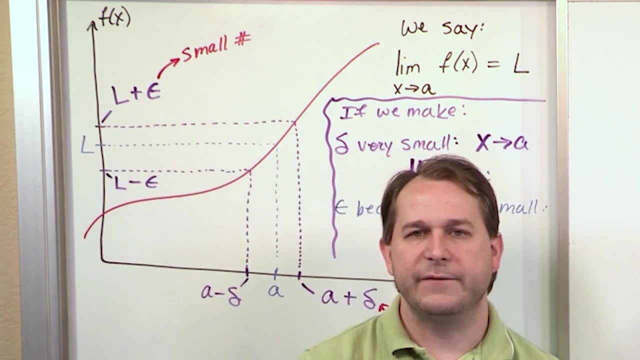 a And as we do that, you can trace your little fingers up and see that the limit is going to approach l, because epsilon is going to get smaller and smaller as you do that. That is essentially the definition of the limit. If you understand that, you can probably stop the video now and 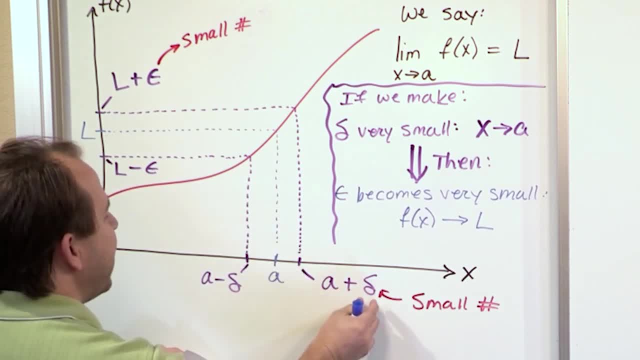 this, and we'll pick a value to the left of this, and the value only differs by this tiny, tiny number that we call delta. both of these points are equidistant on this side to the left and to the right, by a tiny, tiny thing: delta. okay, now, as the drawing stands, these course numbers. 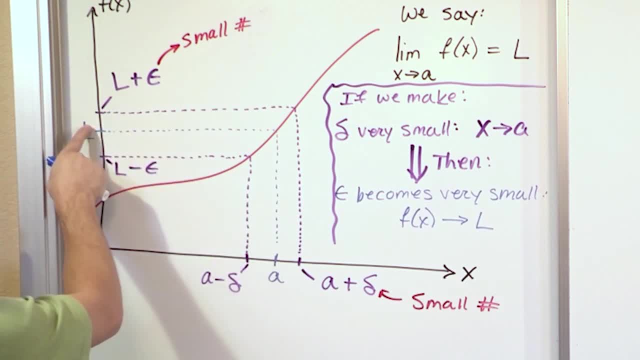 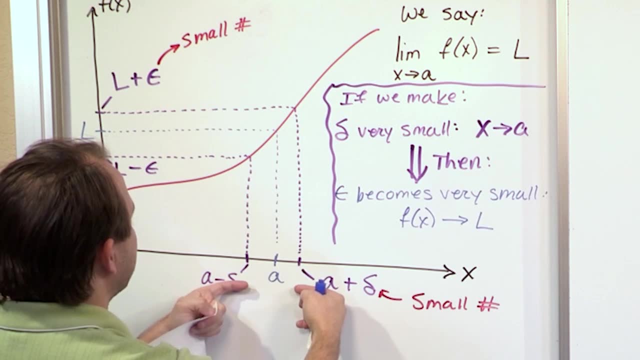 correspond to values up here, one of which is a little bit higher and a little bit lower than the limit that we're seeking, l. but what we're going to do is we're going to make delta get very, very small. so what's going to happen is we're going to encroach closer and closer and closer. 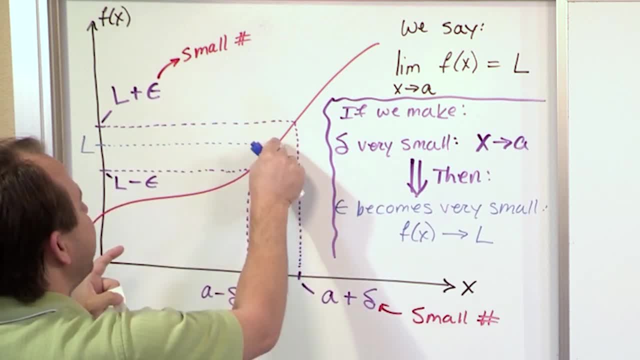 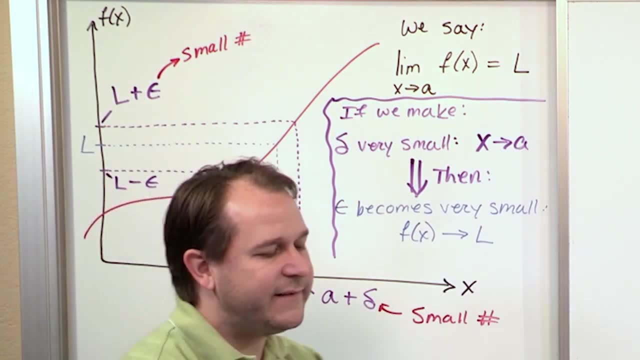 and get infinitely close to a, and as we do that, you can trace your little fingers up and see that the limit is going to approach l, because epsilon is going to get smaller and smaller as you do that. that is essentially the definition of the limit. if you understand that, you can probably 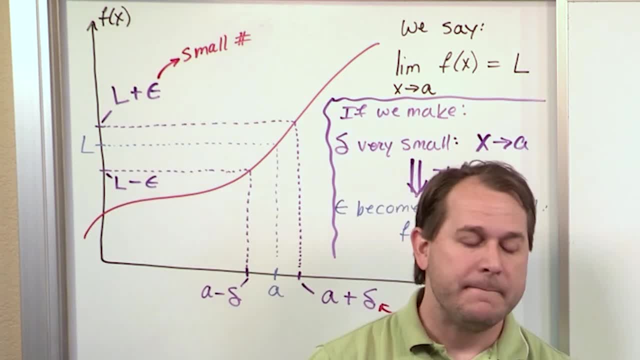 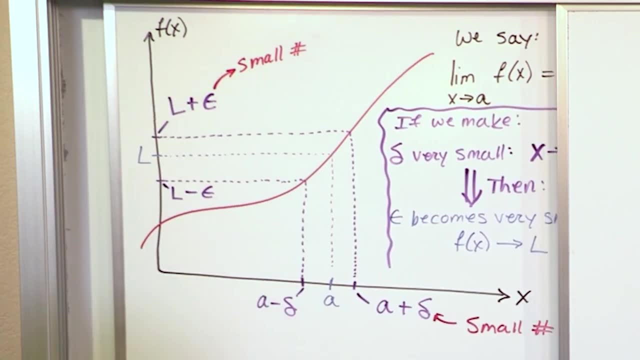 stop the video now and just say that you at least understand what's going on. but let me flip the board back and show you what you're going to read in a typical textbook. okay, so remember that this is what the definition of a limit is. this is what you're. 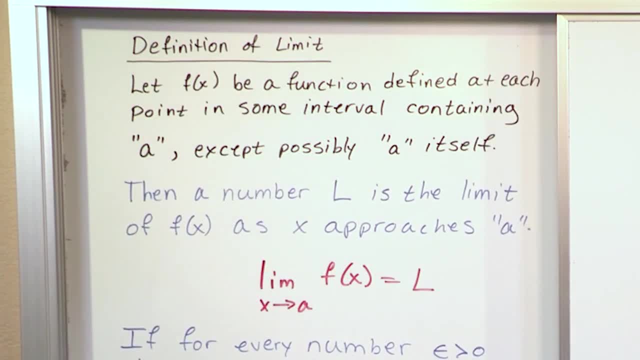 going to read in the textbook. when most student students read this, they're absolutely um. i mean, i know i was dumbfounded when i read. i was like, what does this actually mean? i think i understand limits, but i don't understand this. so this is the definition of a limit. let f of x be a function. 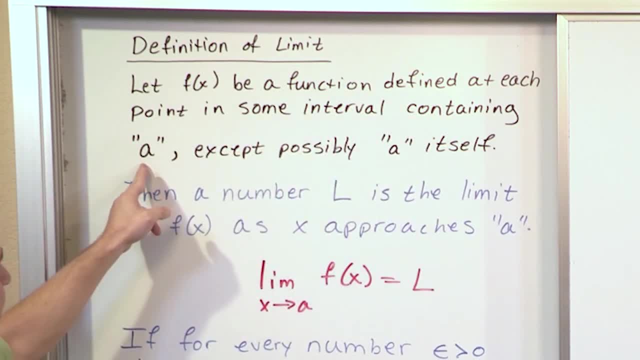 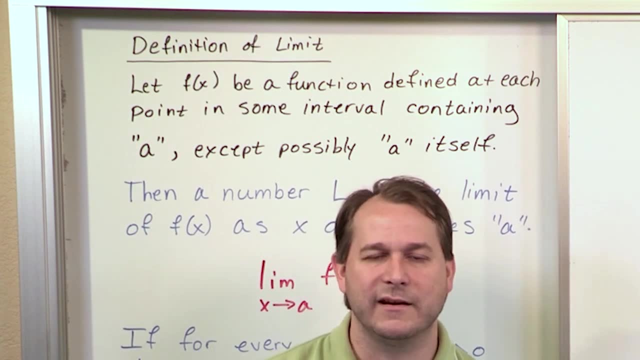 defined at each point in some interval containing a, except possibly a itself, right? so the top part of the definition, if i want to break it down for you all it says is: let f of x be a function defined on an interval that contains some number- a sometimes you may. 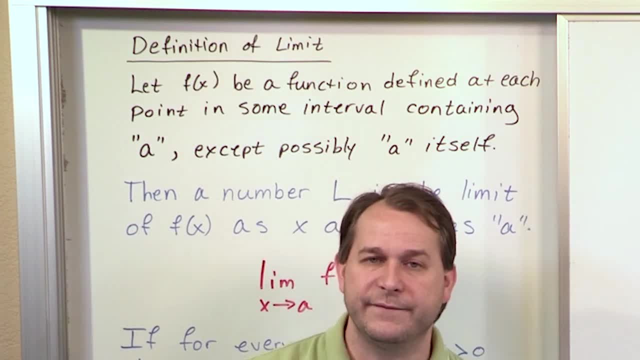 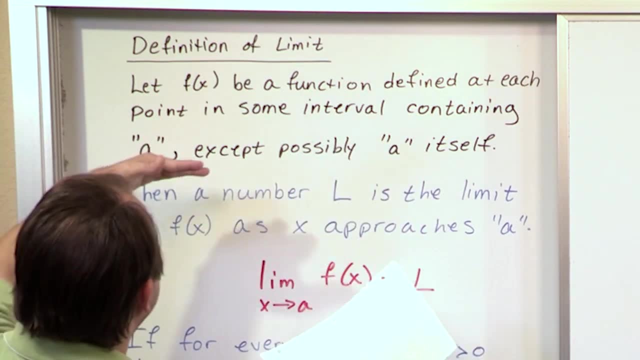 it may not contain the number a, just depending on how your function is defined. okay, because you can have piecewise defined functions in certain intervals. but for the sake of understanding this, just the black text, just tell yourself: okay, all this is saying is that their function exists. 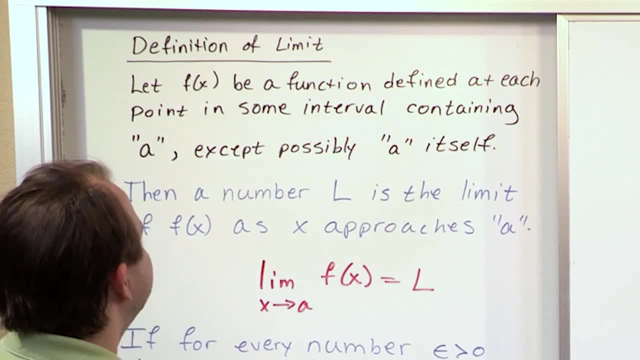 there's a point a inside an interval. that's basically all it says. the definition of the limit is down here. below. it says then a number l is the limit of f of x as x approaches a. in terms of this terminology which we've been writing down, this: 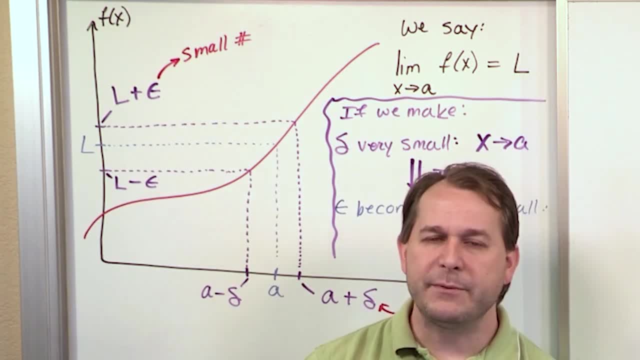 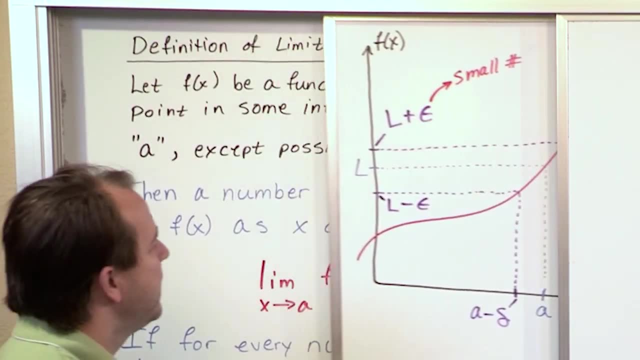 just say that you at least understand what's going on. But let me flip the board back and show you what you're going to read in a typical textbook. Okay, so remember that this is what the definition of a limit is. This is what you're going to read in the textbook When most students read this. 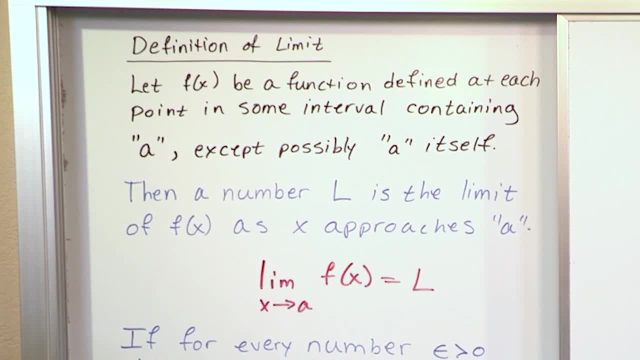 they're absolutely. I mean, I know I was dumbfounded when I read it. I was like, what does this actually mean? I think I understand limits, but I don't understand this. So this is the definition of a limit. Let f of x be a function defined at each point in some. 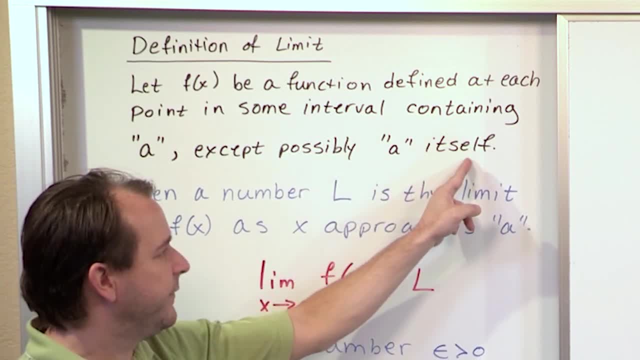 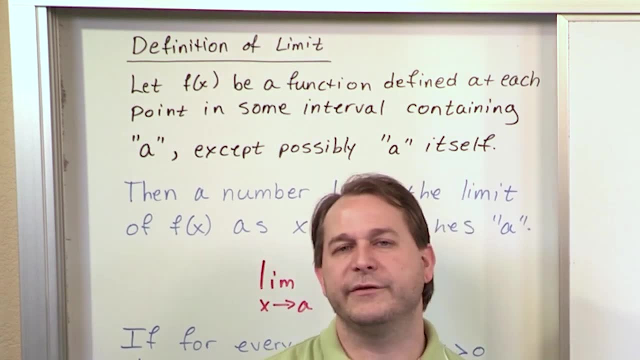 interval containing a, except possibly a itself right. So the top part of the definition. if I want to break it down for you, all it's going to do is it's going to be a function that's going to be defined at each point in some interval. So what it says is: let f of x be a function defined on an. 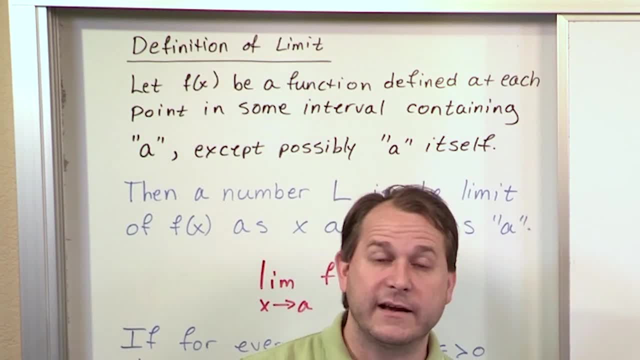 interval that contains some number a. Sometimes it may not contain the number a, just depending on how your function is defined. okay, Because you can have piecewise defined functions in certain intervals. But for the sake of understanding this, just the black text, just tell yourself. 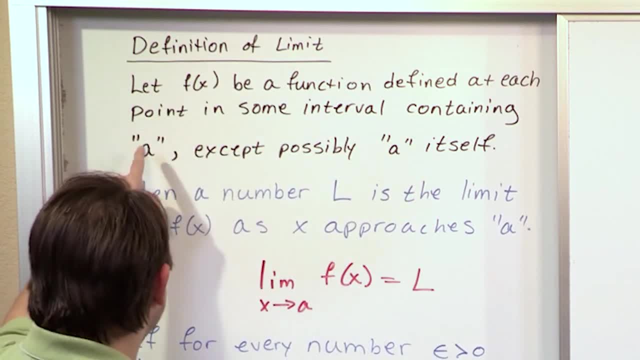 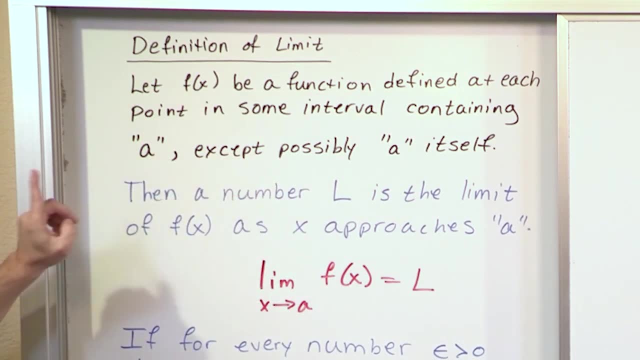 okay. all this is saying is that their function exists. There's a point a inside an interval. That's basically all it says. The definition of the limit is down here below. It says: then a number, l is the limit of f of x as x approaches a. in terms of this terminology which we've been writing down, 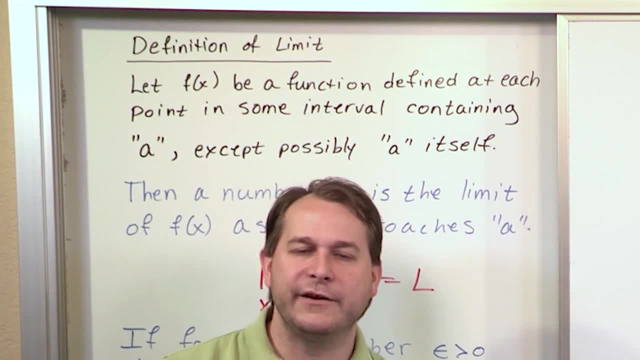 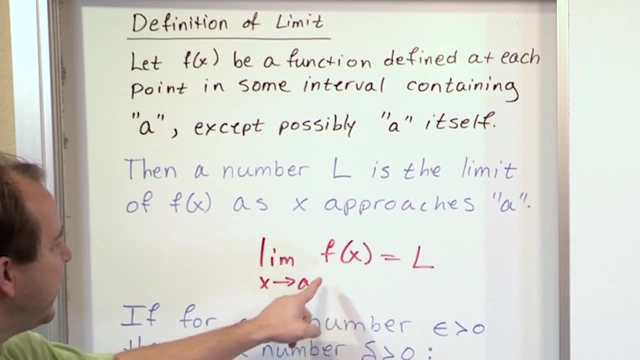 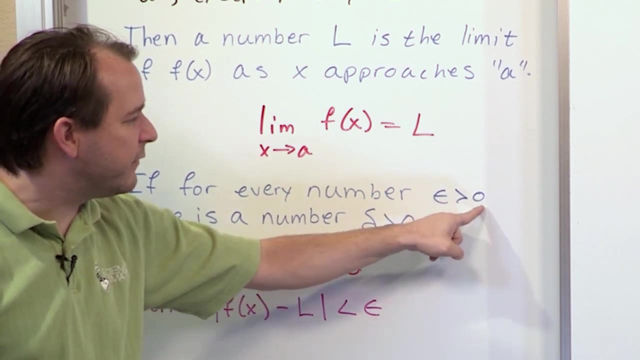 this whole time. okay, Now here's the kicker, here's the punchline, here's the part of it that you wouldn't understand without the drawing before. So this is the limit. as x approaches a of the function becomes l. if, for every number epsilon- that's a positive number- epsilon is greater than. 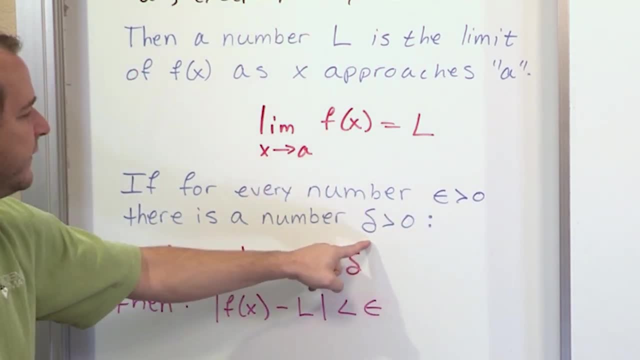 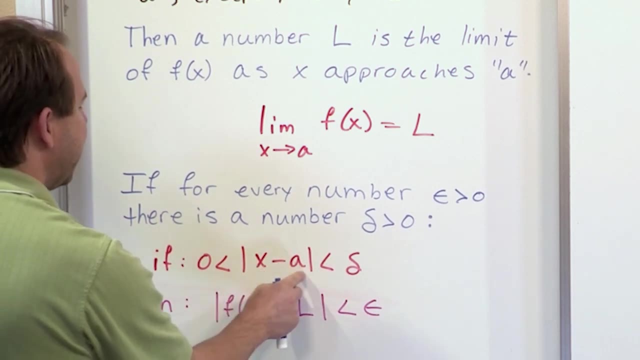 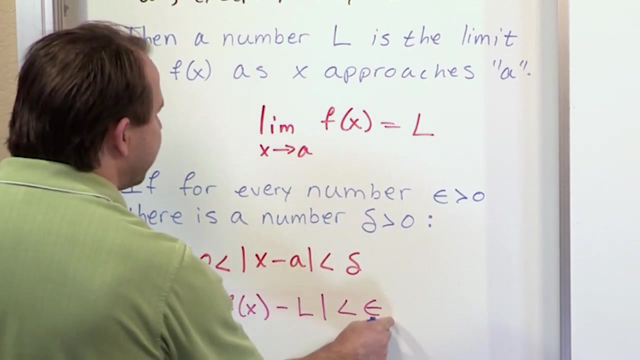 zero, there is a number- delta- that's also a positive number- that satisfies these conditions. What this first one says is: if the difference between x and a is between zero and delta, then the difference between the function and the limit is a very small number, epsilon, You might. 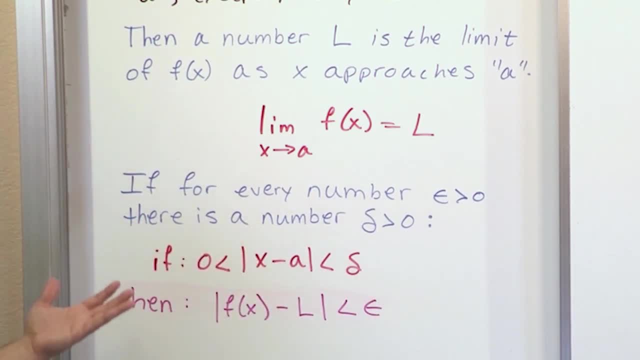 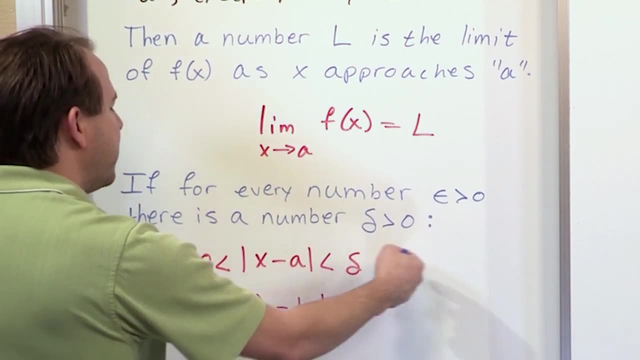 have to read this over and over and over to really understand what it's saying, But in words what's happening is. what it's saying is if I let the difference between x and a become really, really small, what it's saying is, the difference between x and a gets really small because 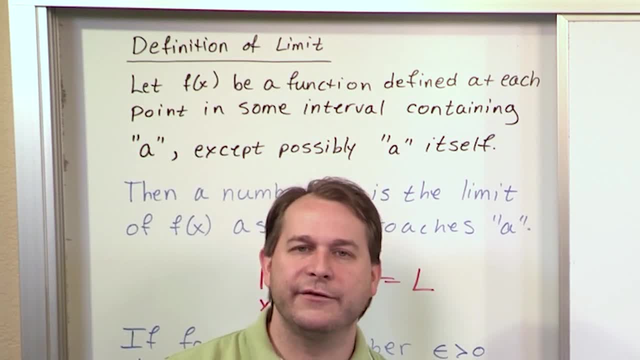 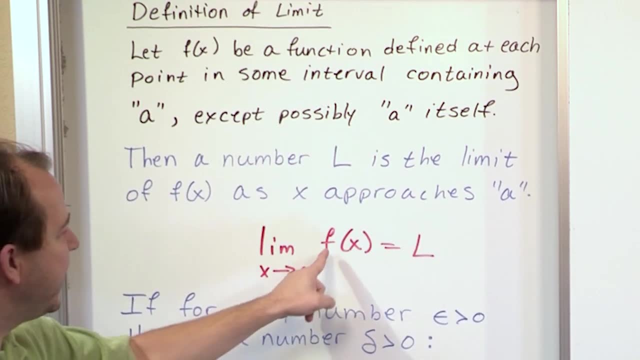 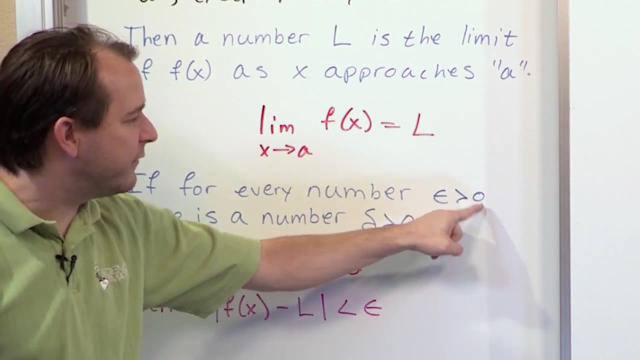 whole time. okay, now here's the kicker, here's the punch line, here's the part of it that that you, you know you wouldn't understand without the drawing before. so this is the limit. as x approaches a of, the function becomes l if for every number epsilon- that's a positive number- epsilon is greater. 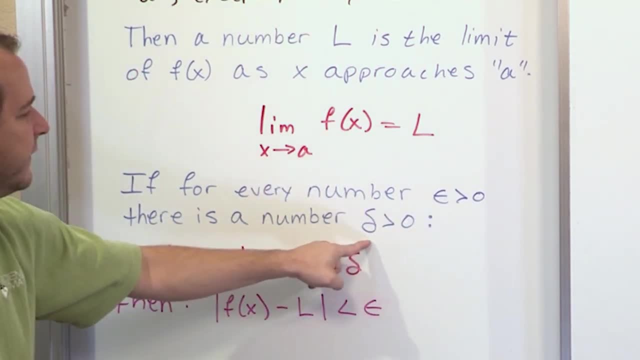 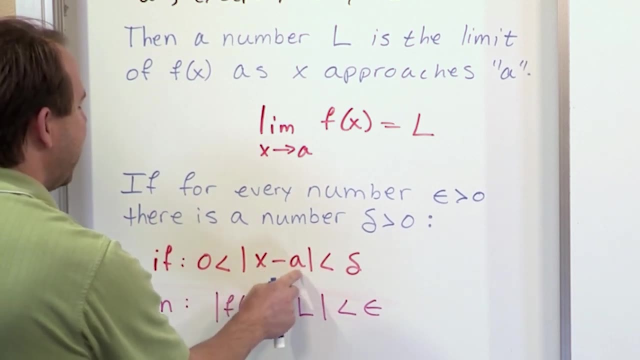 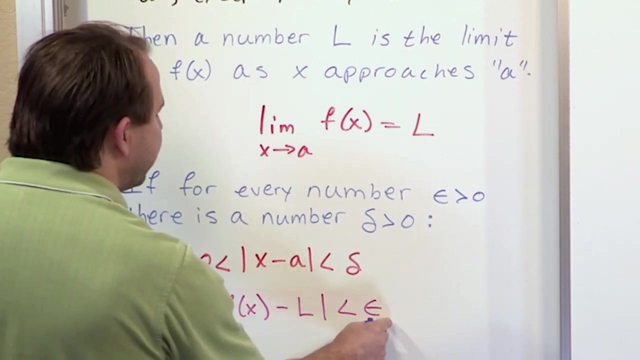 than zero. there is a number- delta- that's also a positive number- that satisfies these conditions. what this first one says is: if the difference between x and a is between zero and delta, then the difference between the function and the limit is a very small number, epsilon. you might have to read this over and over and over to really understand what it's saying. 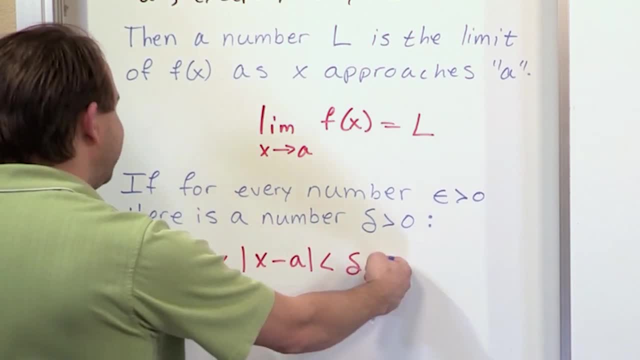 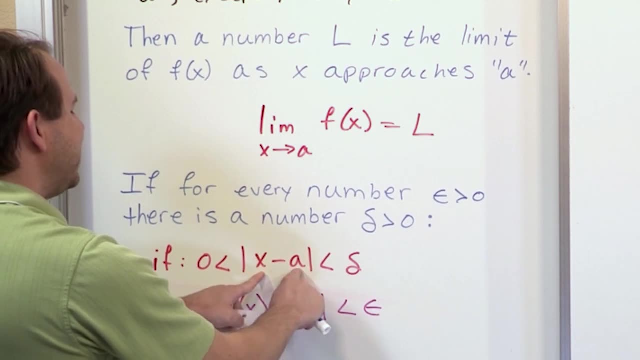 but in words, what's happening is what it's saying is, if i let the, if i let the difference between x and a become really really small, what it's saying is the difference between x and a gets really small because, remember, delta is a small number. i told you that delta is an incredibly small number. 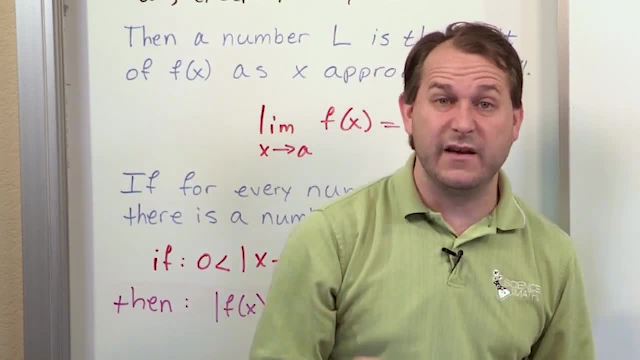 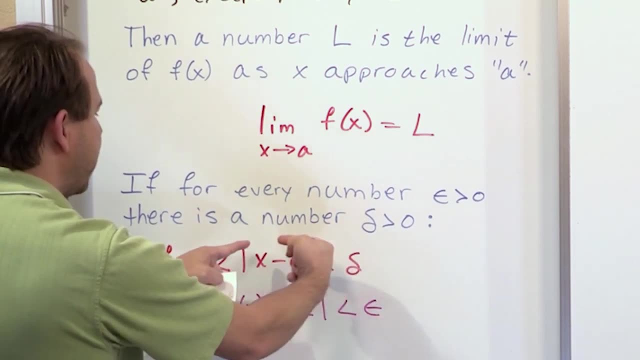 it's like maybe infinitesimally small number. that's what delta is. so what i'm saying is, if i let my variable x, the difference between x and a is the distance. you know, i'm approaching x, right? so if i'm tracing my finger along the difference between x and a, if it becomes a really small, 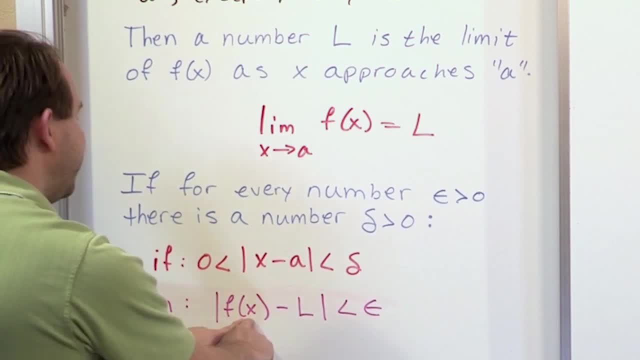 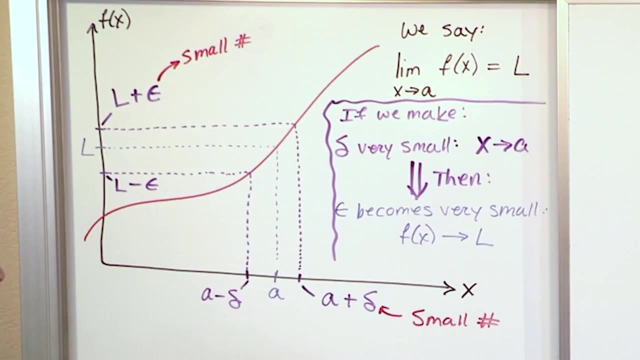 number between zero and delta, then the difference between the function and the limit is going to be a very, very small number. that's exactly what i told you 25 times a second ago. what i'm saying is, as you trace your fingers left and right, every point you have your fingers, there's a distance. 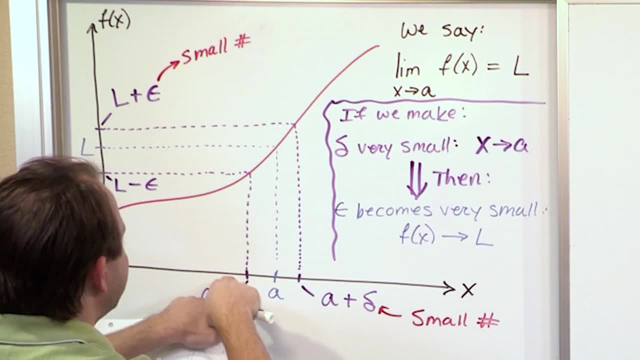 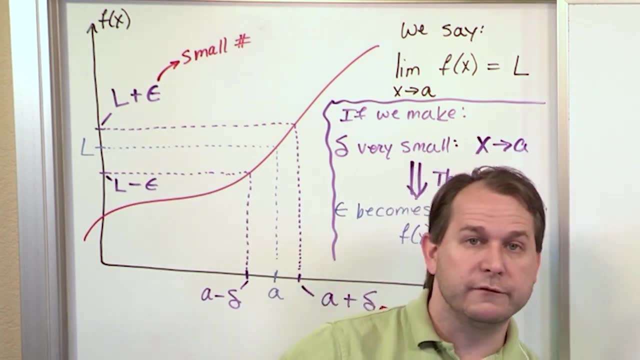 between the value you have and a. okay, we do that as we make our tables, remember, we plug in values farther away and then closer and closer and closer and closer. right, so the difference between my finger and a? okay, if i let that get really small, if the difference between x and a is really small, 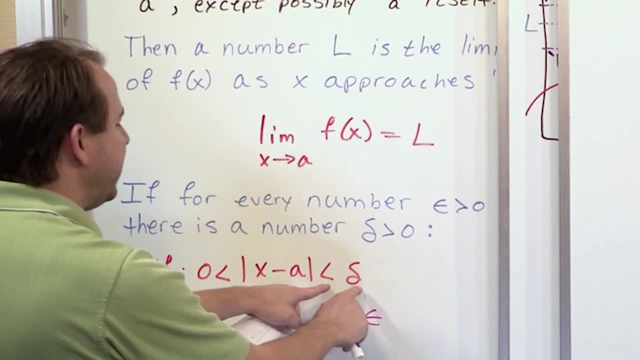 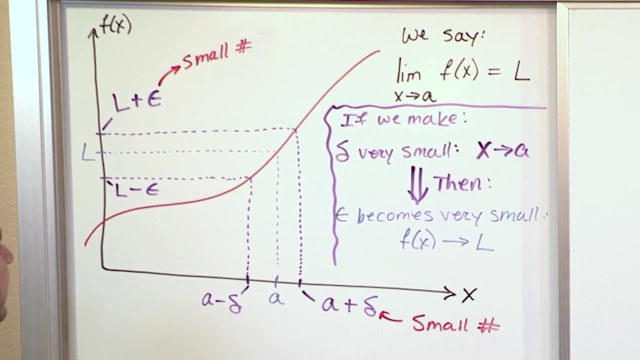 then the difference between x and a is going to be a very, very small number, and the difference between x and a gets really small, which means this difference here is between zero and an incredibly tiny number, delta. all that is saying is that my finger is very, very, very, very, very very. 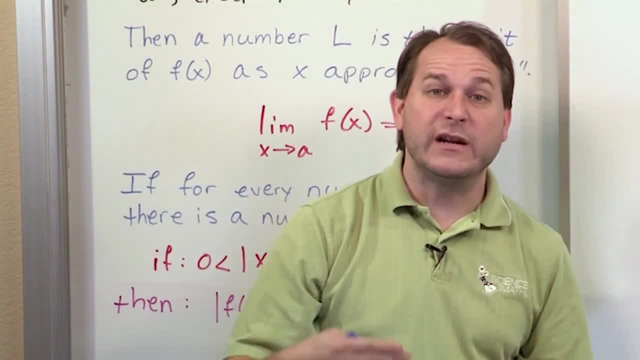 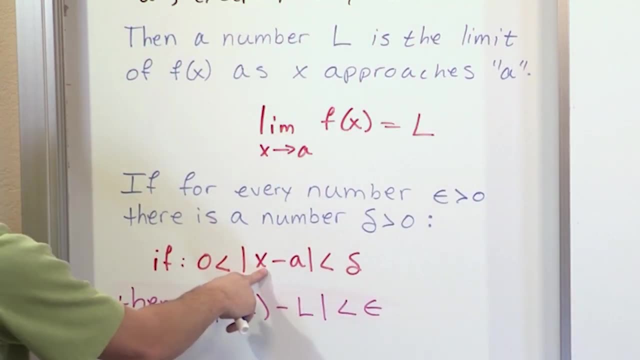 because, remember, delta is a small number. I told you that Delta is an incredibly small number. It's like a itty bitty, bitty, infinitesimally small number. That's what delta is. So what I'm saying is, if I let my variable x 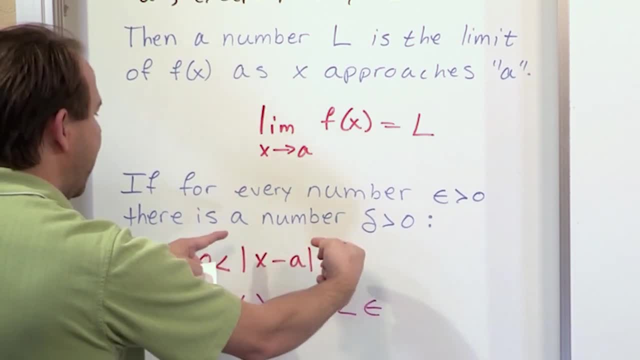 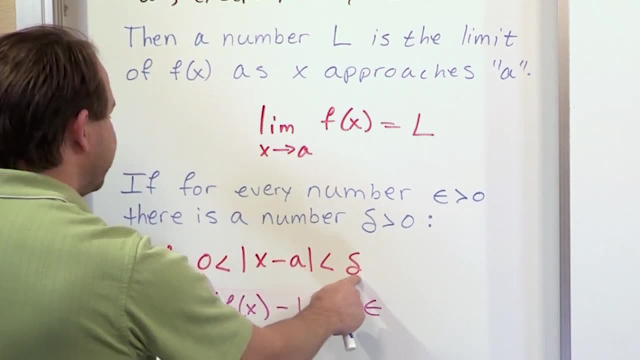 the difference between x and a is the distance. you know I'm approaching x, right? So if I'm tracing my finger along the difference between x and a, if it becomes a really small number between zero and delta, then the difference between the function and the limit. 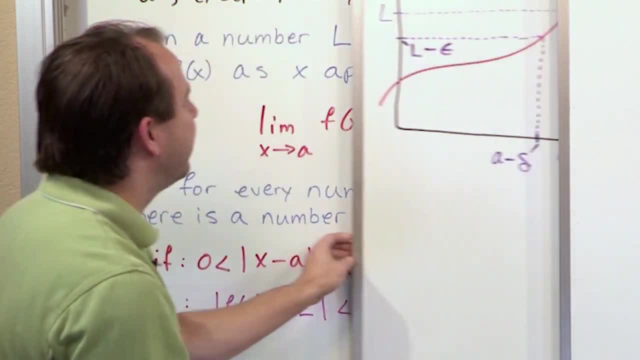 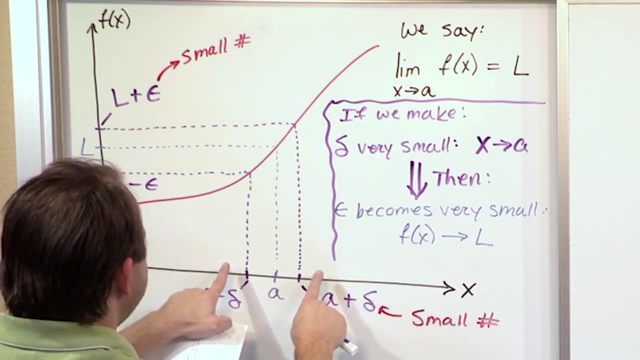 will be a very, very small number. That's exactly what I told you 25 times a second ago. What I'm saying is, as you trace your fingers left and right, every point you have your fingers, there's a distance between the value you have and a okay. 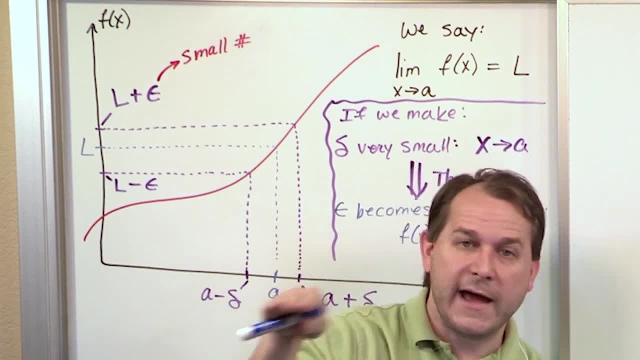 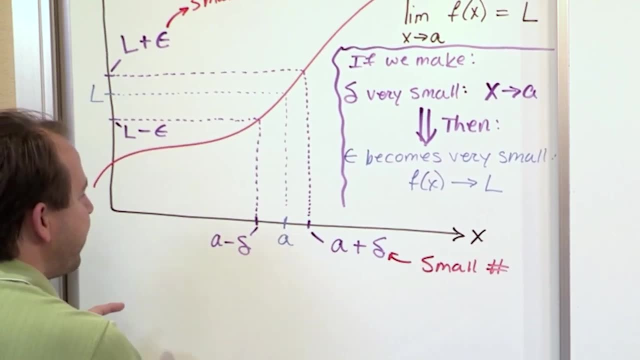 We do that as we make our tables, Remember, we plug in values farther away and then closer and closer and closer and closer. right So the difference between my finger and a. okay, If I let that get really small, if the difference between x and a gets really small, 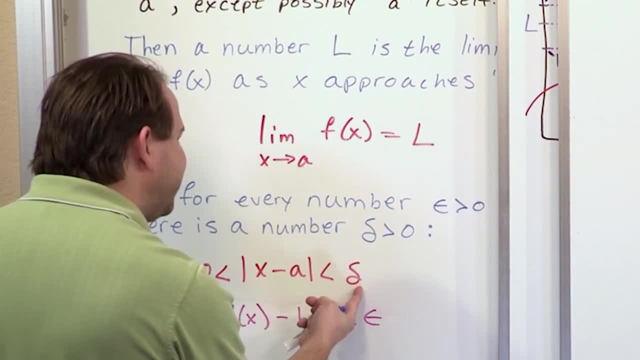 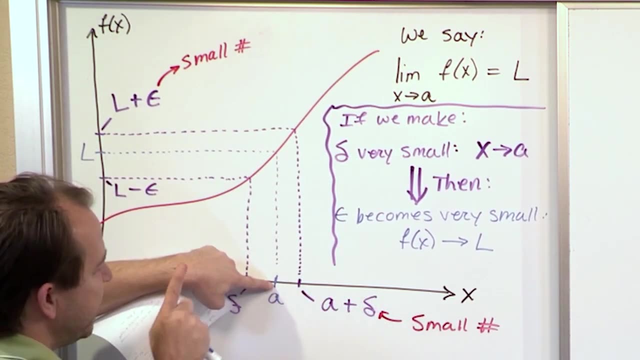 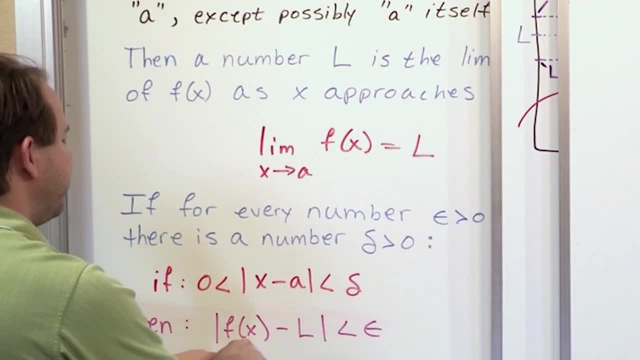 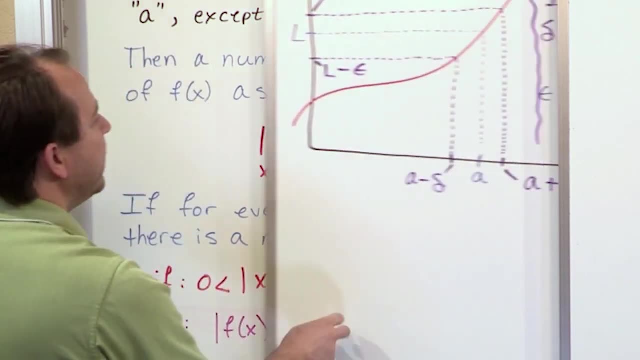 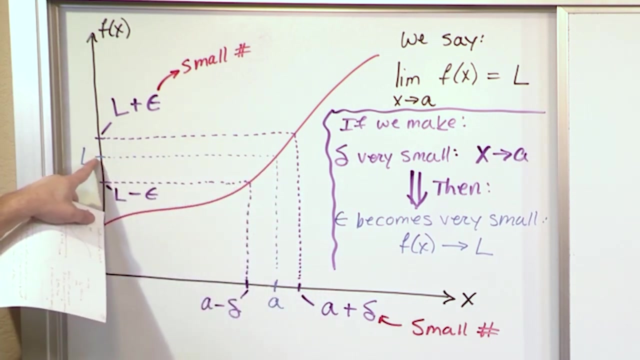 Then, if I let this happen, then the difference between the function and the limit l is also gonna be a really, really, really small number. okay, All it's saying is that as my finger gets infinitely close to a, then the function gets infinitely close to l. 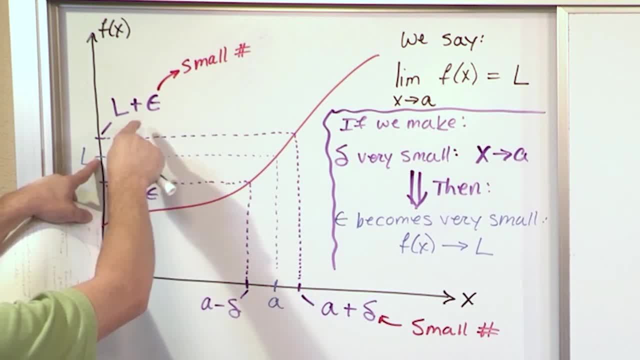 because it differs. the difference between the function and the l differs by a very small number. All it's saying is that as I squeeze my fingers this way, then this becomes squeezed together as well. The reason there's absolute values here is because of the way I've drawn the picture. 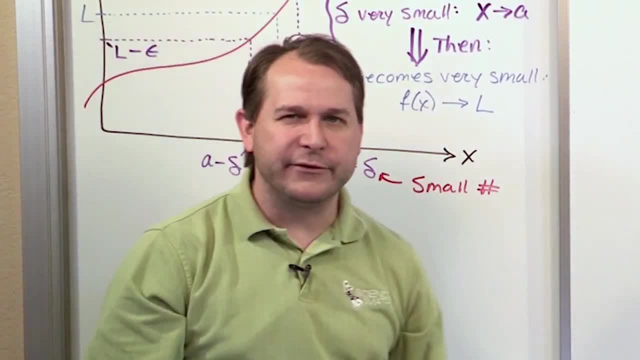 because I can approach from the left or I can approach from the right. Remember the absolute value. all it does is it just throws away the sign. Doesn't matter if you're coming from the left or if you're coming from the right. 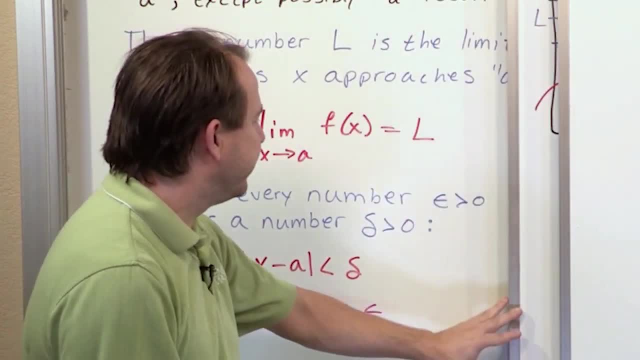 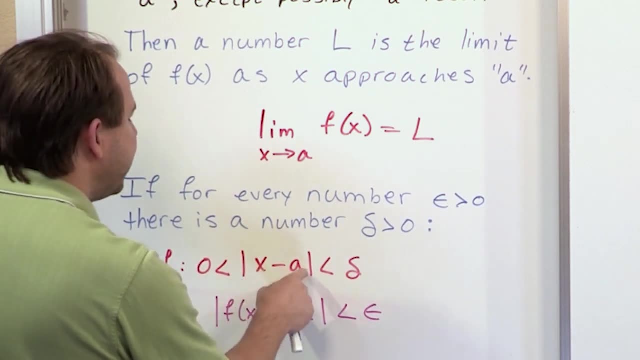 it throws away the sign. So that's why those absolute values are there, because it doesn't matter if I'm approaching from the left of a or from the right of a, It doesn't matter if x minus a is positive or if x minus a is negative. 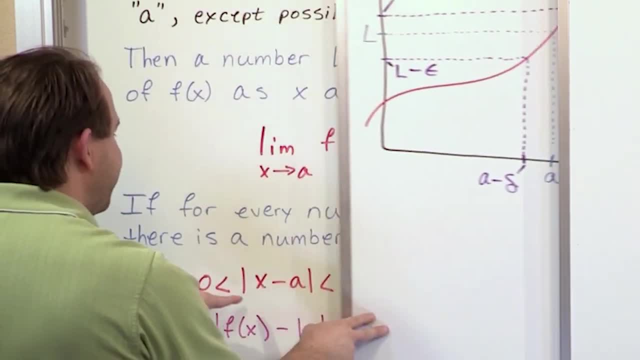 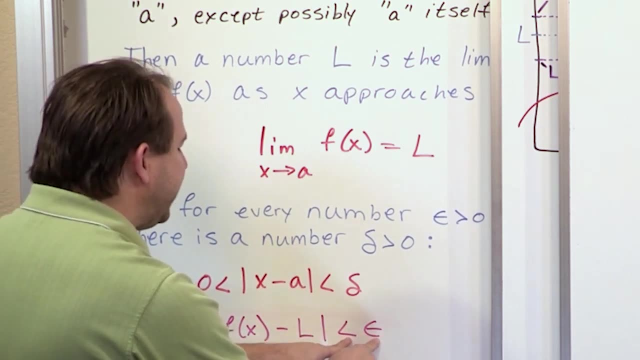 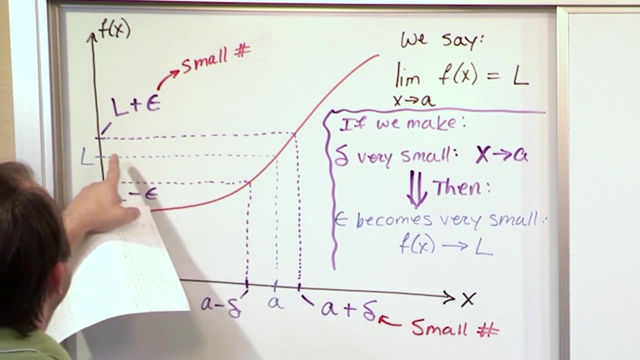 very, very, very close to a, but it never quite gets there. then if i let this happen, then the difference between the function and the limit l is also going to be a really, really, really small number. okay, all it's saying is that as my finger gets infinitely close to a, then the function 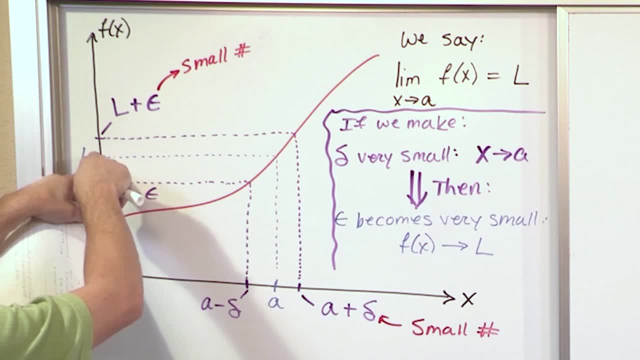 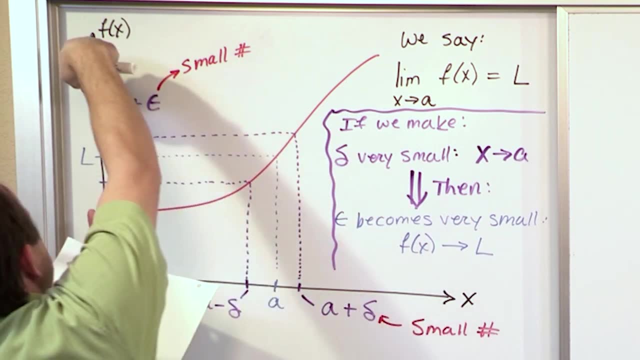 gets infinitely close to l because it differs. the difference between the function and l differs by a very small number. all it's saying is that as i squeeze my fingers this way, then this becomes squeezed together as well. the reason there's absolute values here is because of the way i've 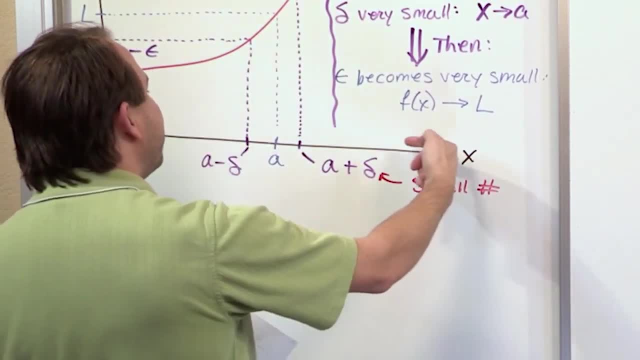 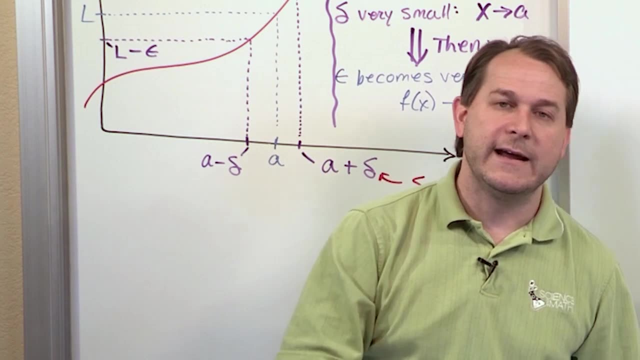 drawn the picture because i can approach from the left or i can approach from the right. remember the absolute value. all it does is it just throws away the sign. doesn't matter if you're coming from the left or if you're coming from the right, it throws away the sign. so. 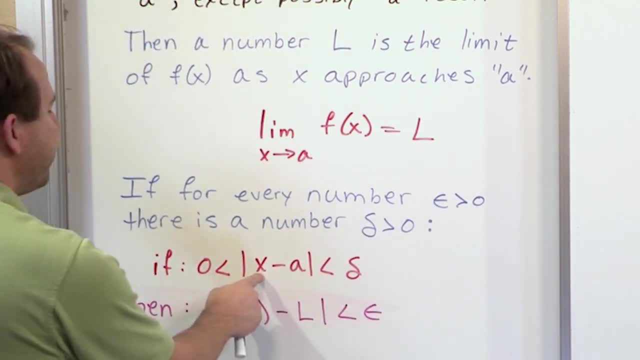 that's why those absolute values are there, because it doesn't matter if i'm approaching from the left of a or from the right of a. it doesn't matter if x minus a is positive or if x minus a is negative. i'm approaching from the other way, whatever the difference is. i just look at the absolute value. 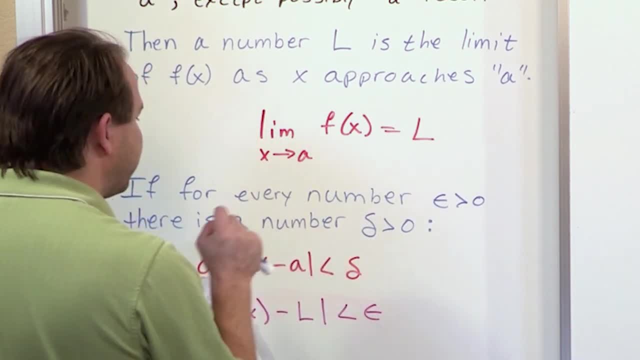 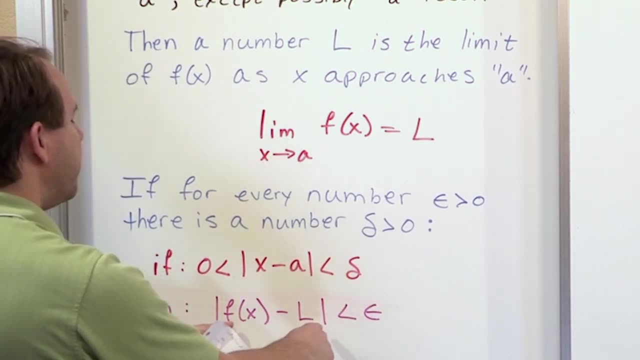 and it's going to be a very small number because it's between zero and delta, which is incredibly tiny. okay, when this happens, the function itself approaches the difference between the function and l approaches a very, very, very small value, or it's less than a very, very 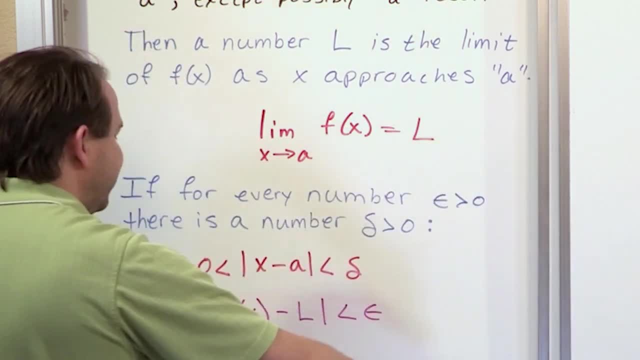 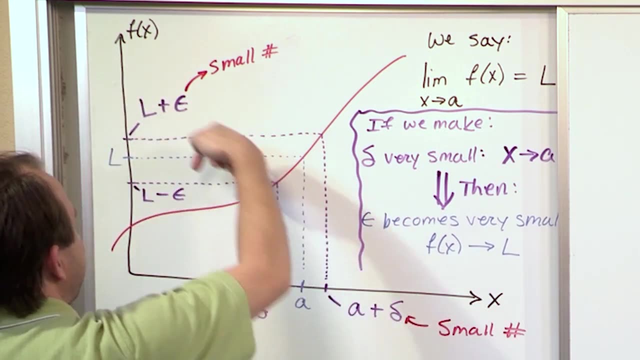 small value. it doesn't matter if i'm approaching from the top or the bottom. see, this is f of x minus l, f of x minus l. when if i'm approaching from this way, like if i'm coming this way, f of x minus l will be positive, because this number minus this number is positive. but if i'm coming, 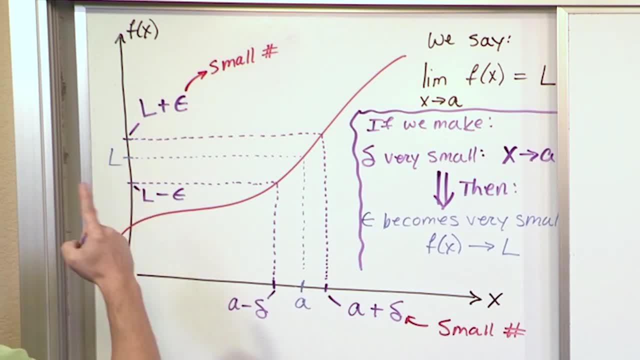 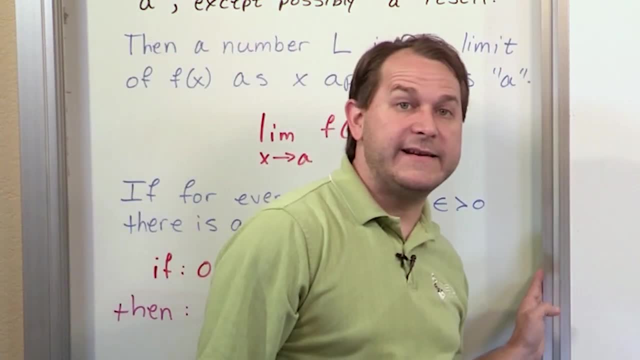 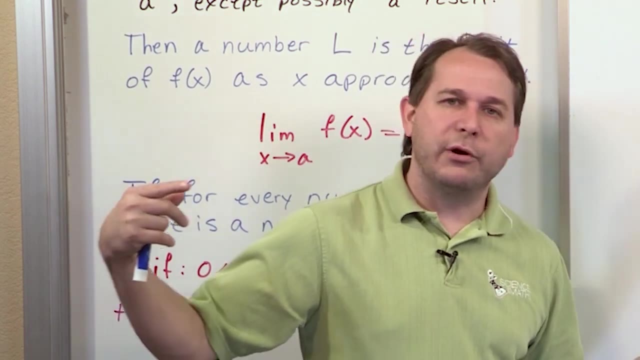 this way then this number f of x minus l will be negative. but you see, the absolute value throws a sign, just throws it away. so the only reason we have absolute value signs in that definition is because it doesn't matter if you approach from the underside, from the left hand side, to find the limit, or if you approach from the right hand side to find the. 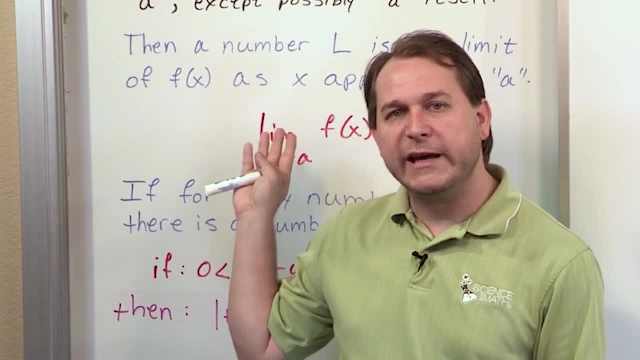 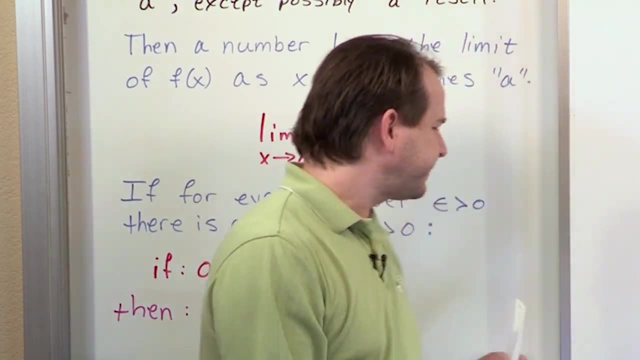 limit. okay, that's the bottom. that's the bottom line is, whenever we're looking at a limit at a point like that, okay, then we basically want to be able to come from the left or from the right, and what's happening here is that if we get infinitely close to this point, 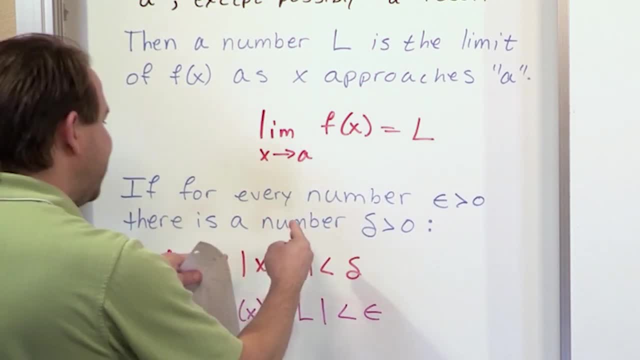 I'm approaching from the other way. Whatever the difference is, I just look at the absolute value and it's gonna be a very small number because it's between zero and delta, which is incredibly tiny. okay, When this happens, the function itself approaches. 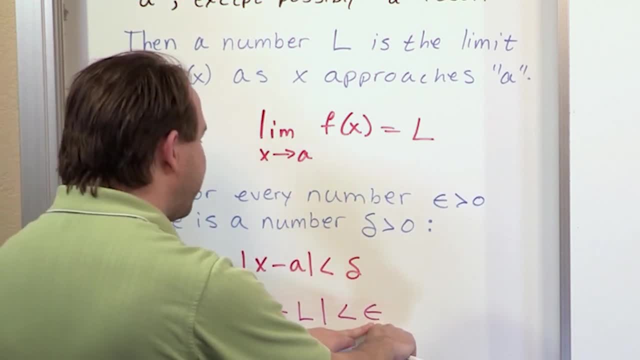 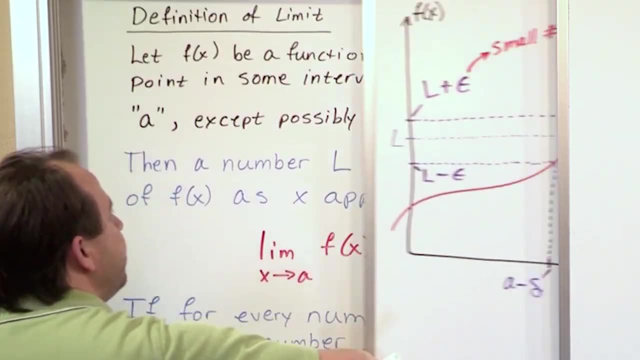 the difference between the function and l approaches a very, very, very small value, or it's less than a very, very small value. It doesn't matter if I'm approaching from the top or the bottom. See, this is f of x minus l. 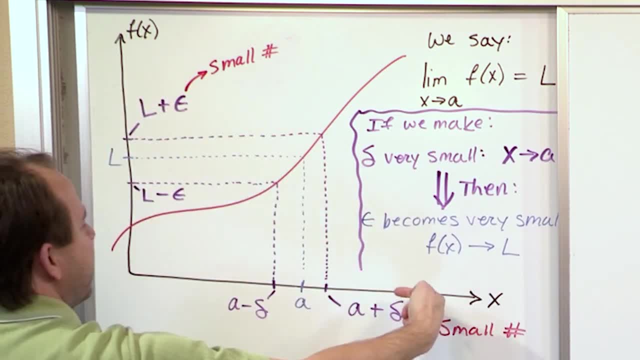 f of x minus l. if I'm approaching from this way, like if I'm coming this way, f of x minus l will be positive, because this number minus this number's positive, But if I'm coming this way, then this number f of x minus l, will be negative. 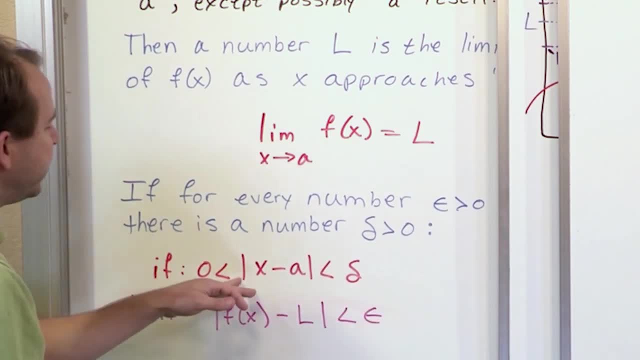 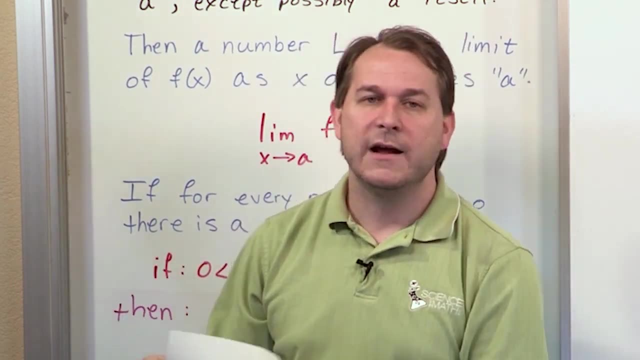 but you see, the absolute value sign just throws it away. So the only reason we have absolute value signs in that definition is because it doesn't matter if you approach from the underside, from the left-hand side, to find the limit, or if you approach from the right-hand side. 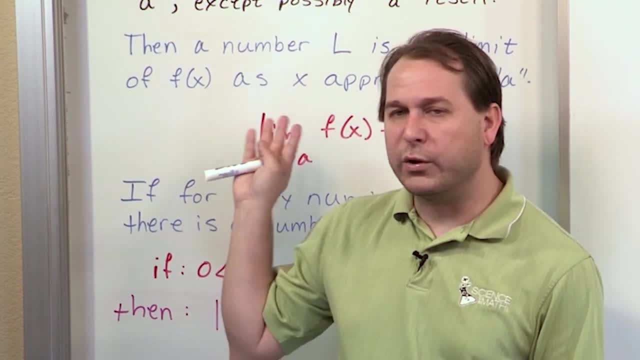 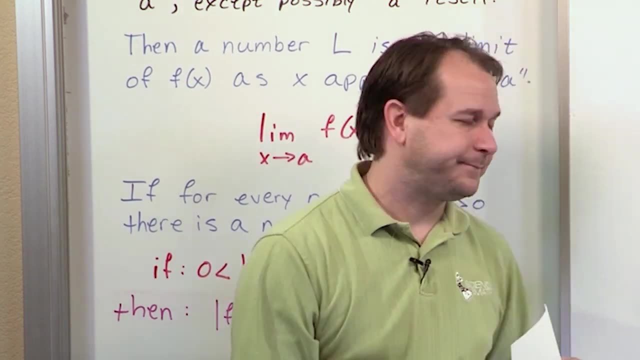 to find the limit. Okay, that's the bottom line- is, whenever we're looking at a limit at a point like that, okay, then we basically want to be able to come from the left or from the right, And what's happening here is that if we get infinitely close, 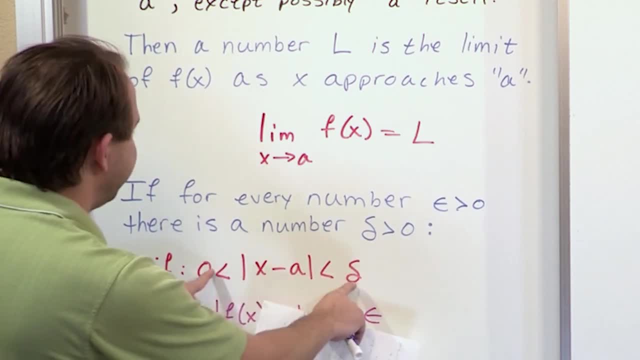 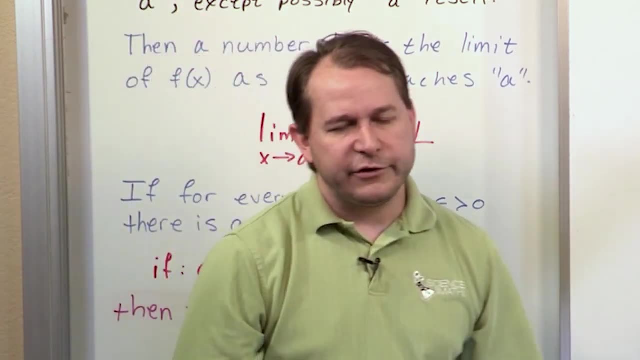 to this point a, which means the difference between the point and a is very, very small, then the difference between the function and the limit approaches this very, very, very small value. There you have it. okay, It's basically it. 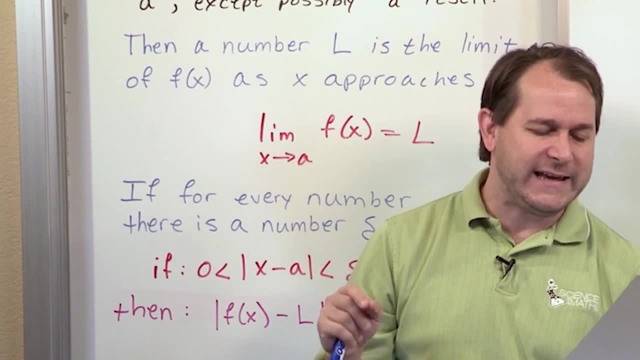 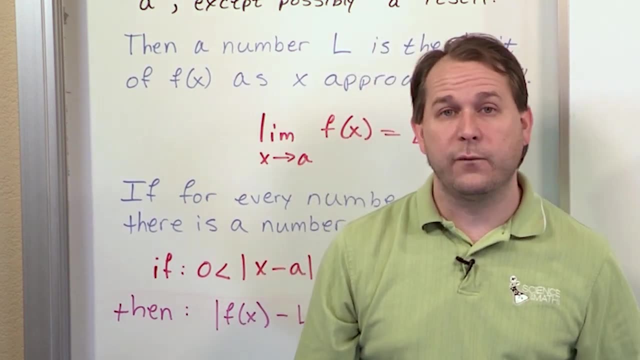 We can let f of x get as close as we want to l by taking x closer and closer to a, but never quite equaling a. Now I told you that in the very first section of what is a limit. okay, I mean, that's what I'm here for. 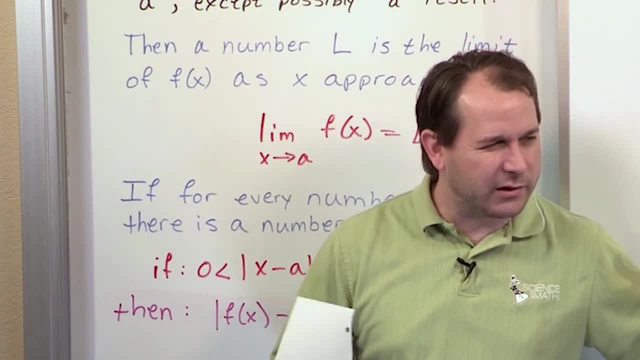 so trying to break it down for you, That's the bottom line. I told you from the very first day that you get closer and closer and closer to l, and then the function gets closer and closer. I'm sorry, let me start over. 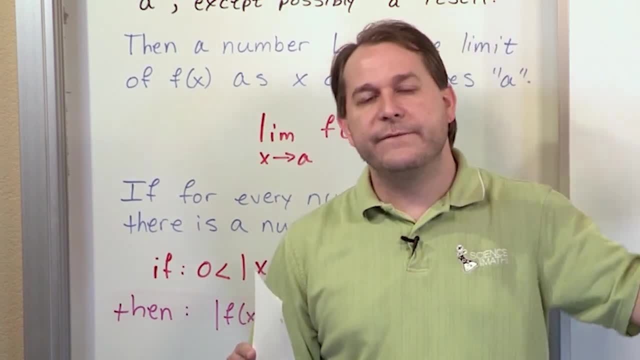 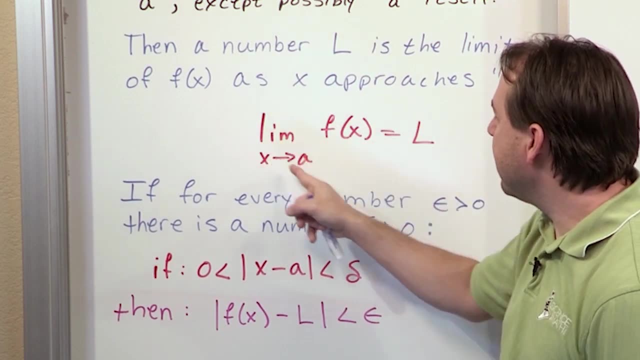 You get closer and closer and closer to a along the axis, and then the function approaches closer and closer and closer to l. This is the mathematical framework that does that. We write the limit down like this. This business, you really never use it practically. 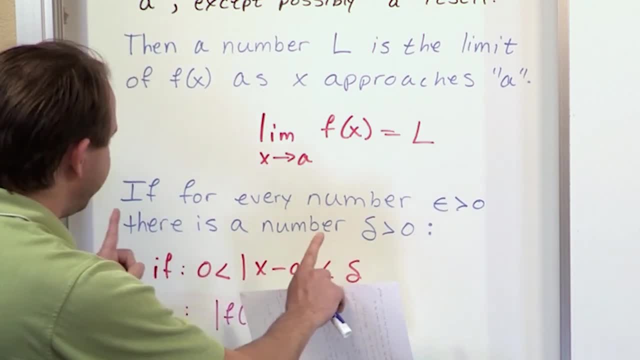 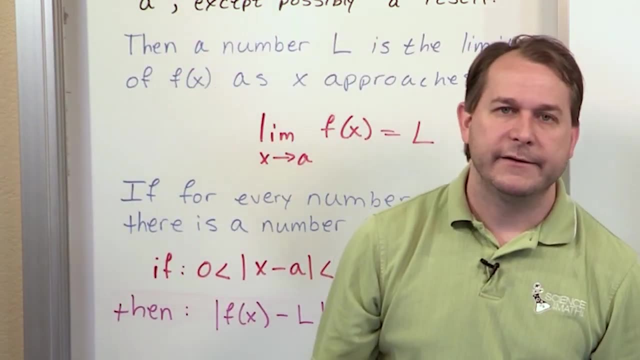 a, which means the difference between the point and a is very, very small. then the difference between the function and the limit approaches this very, very, very small value. there you have it. okay, that is basically it. we can let f of x get as close as we want to l. 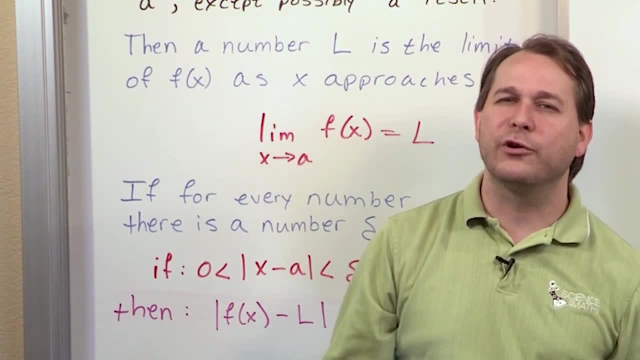 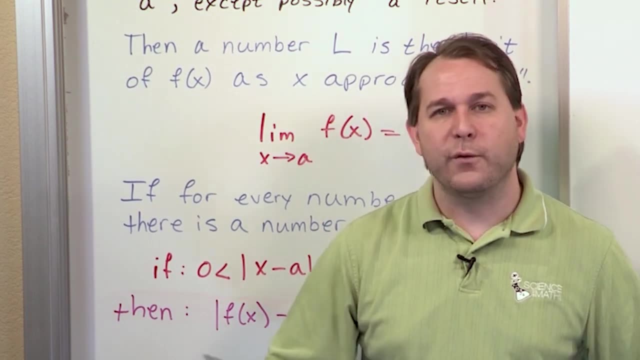 by taking x closer and closer to a, but never quite equaling a. now i told you that in the very first section of what is in limit. okay, i mean, that's what. that's what i'm here for. so trying to break it down for you, that's the bottom line. i told you from the very first day that you 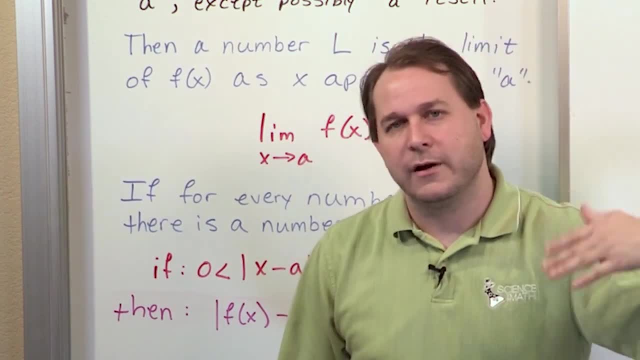 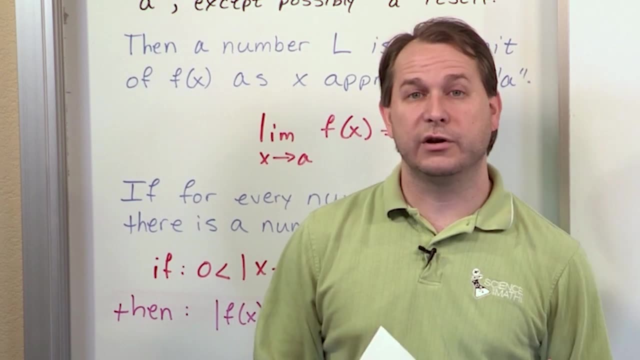 get closer and closer and closer to l, and then the function gets closer and closer. i should- i'm sorry, let me start over. you get closer and closer and closer to a along the axis, and then the function approaches closer and closer and closer to l. this is the mathematical framework that does. 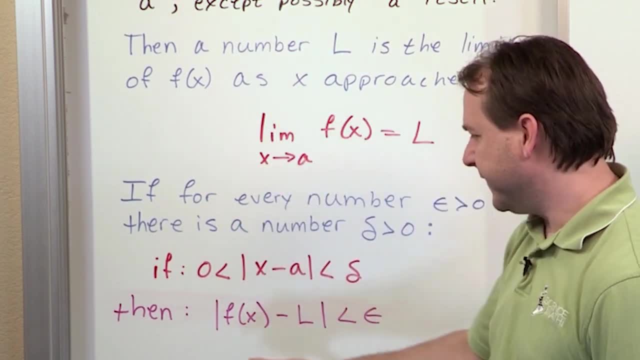 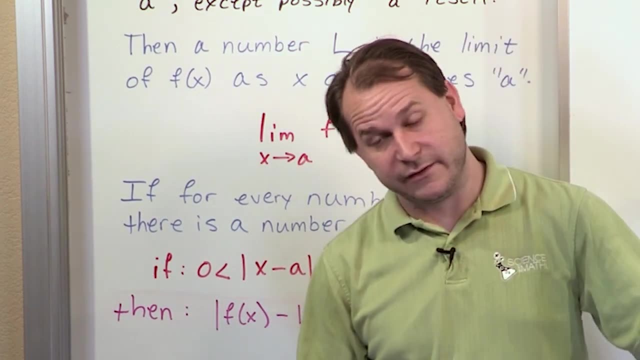 that we write the limit down like this. this business, you really never use it practically. it's just defining what the limit does. it's just saying, hey, if you get closer and closer and closer, then the limits can. the function is going to get closer and closer, closer to the limit, that's all. 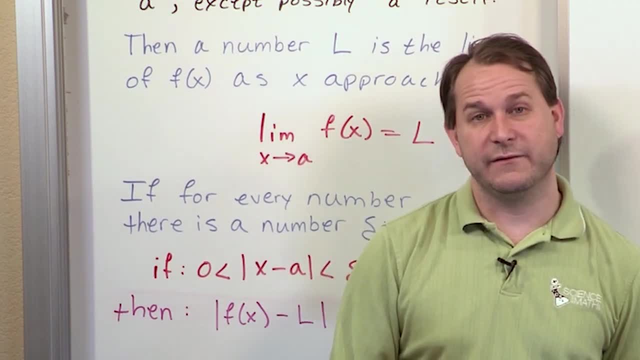 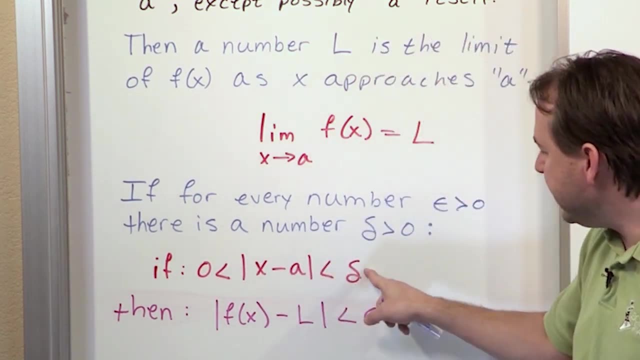 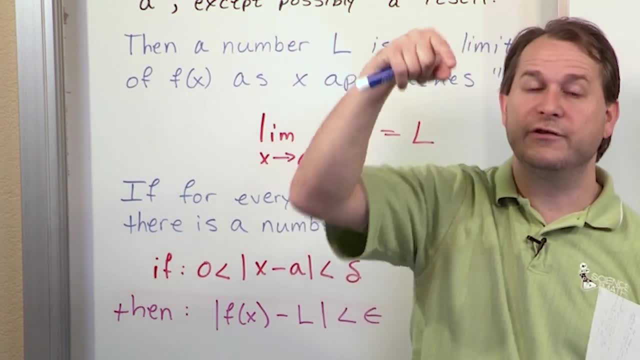 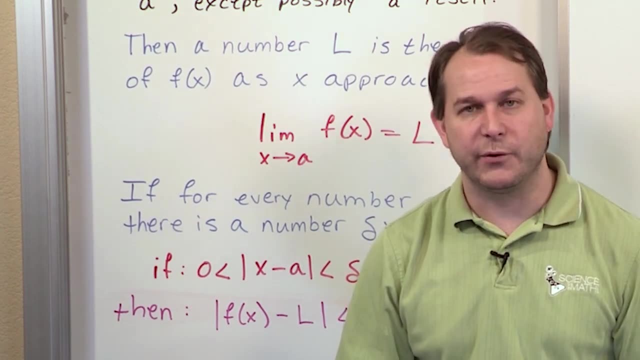 And all it's saying is that if I approach along the axis here, then the function is going to approach that limit. That's all it's saying. So there's no problems for this section. This is mostly just an informational session for you, so you understand what this definition is. 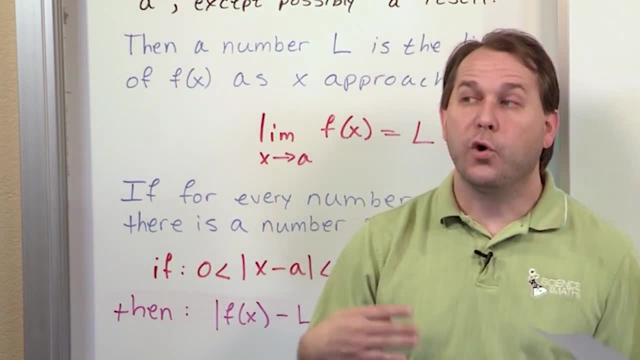 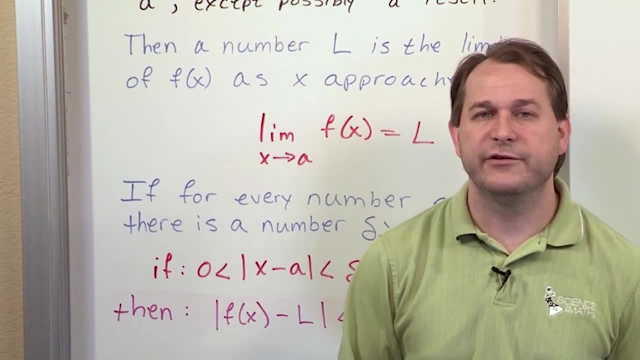 And as you move on to other sections, you'll understand in your back pocket, formally, mathematically, what it means. It's also good practice, now that you understand this, to help you read these types of theorems and definitions and calculus. 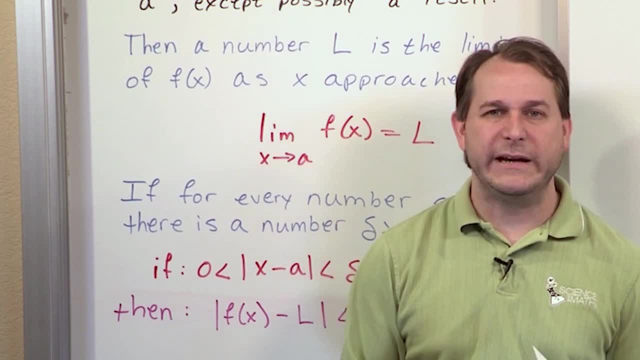 because there'll be more as time goes on and you'll kind of get a little practice reading one of these guys. If you can understand this one, then you can understand any theorem in a calculus book, because this is kind of one of the more difficult ones to understand. 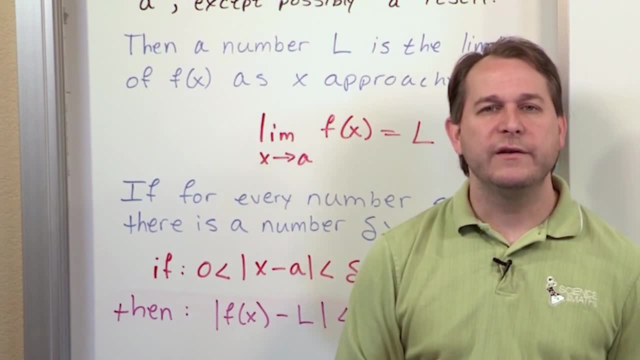 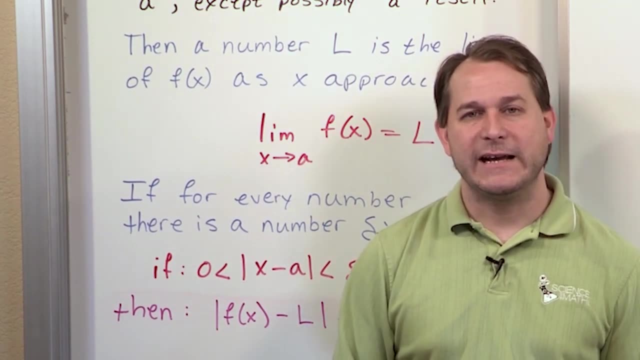 All right, so make sure you understand this and then follow me on to the next section. We're going to talk about something called limit laws or limit rules, and it's going to help you solve different types of limits in calculus. Learn anything at mathandsciencecom.